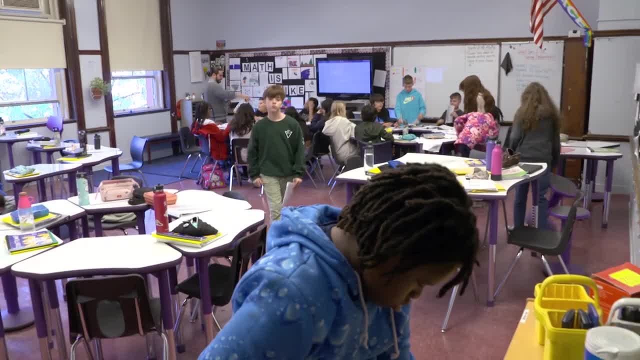 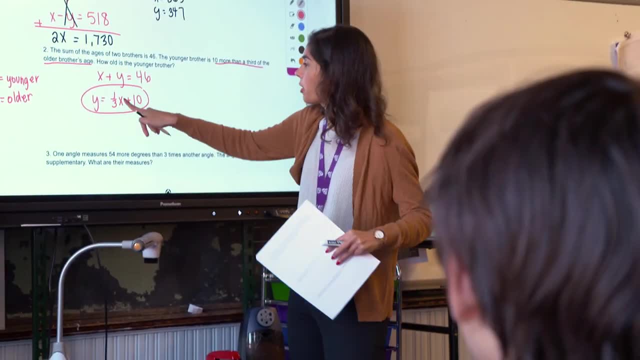 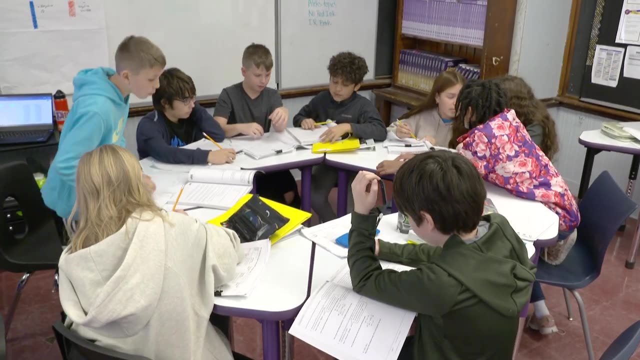 three math teachers And throughout the year we might all teach them. It's all based on where they're at and what they need. Elementary school does like really big lessons, Like I can't focus whenever I'm doing that, But small groups always helps me because I like just I like to engage. But 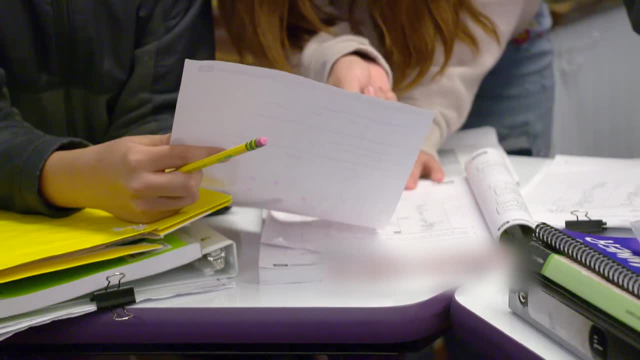 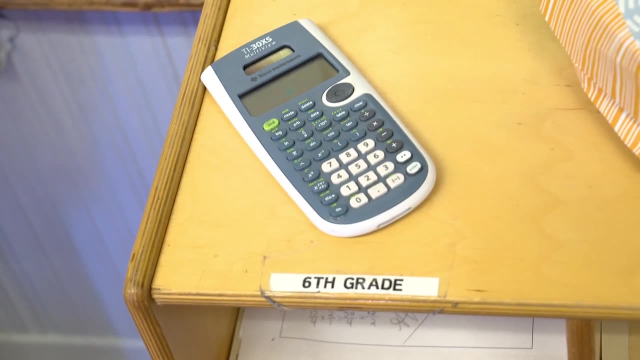 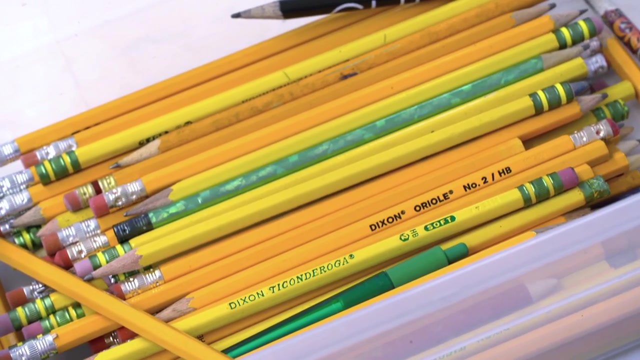 not all the time. you can engage in a big group. Improving students' academic achievement is of critical need and high priority for Illinois. A grade six student actually had the lowest proficiency rate among all the grades that are tested on the state standard test. 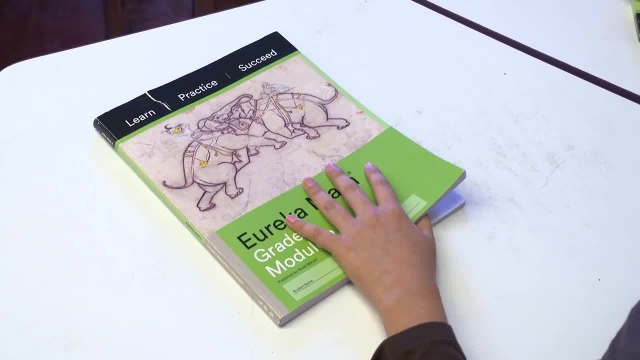 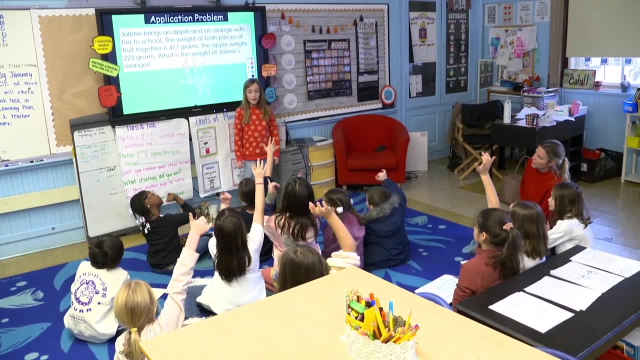 So obviously the grade six is of critical need of support around this. In my experience in elementary school classrooms, usually most students are reasonably engaged in math. Obviously there's some that like it more than others, but there isn't as strong a division of I like math. 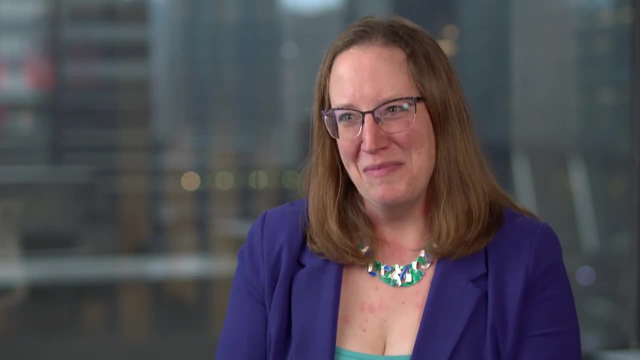 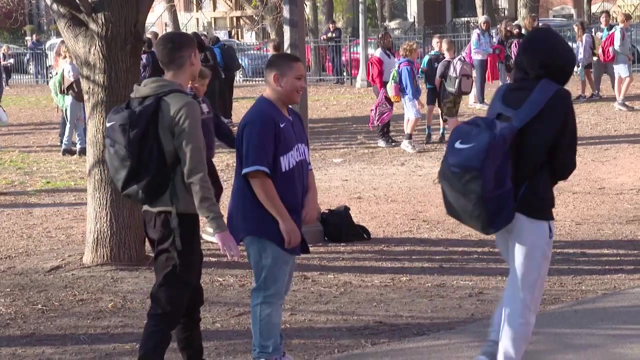 or I don't like math. when I talk to kids, That starts to change in middle school. Middle school is an interesting time in a child's life, I would say. no one ever says, gee, I wanna go back and do middle school again. 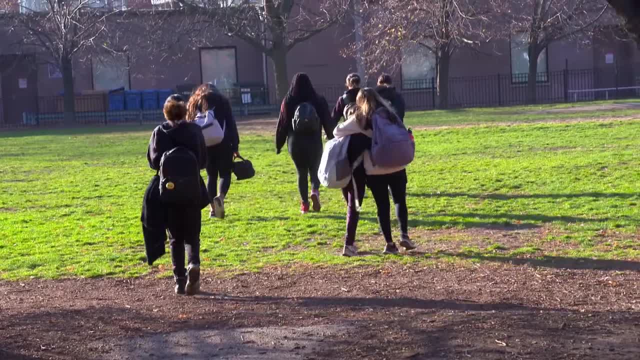 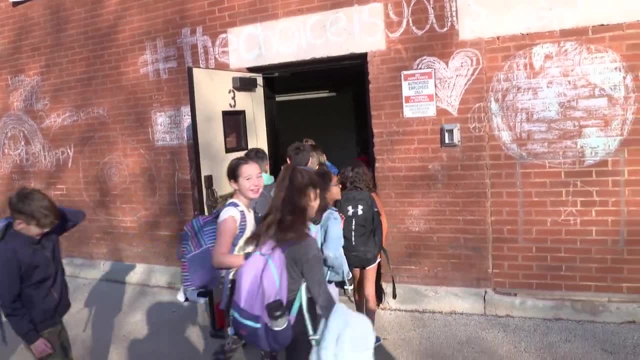 because there's awkwardness. there's the whole social network that you're trying to navigate and everything else. For many years, being good at math was perhaps what put you in the unpopular crowd. So I think students have to like kind of navigate. 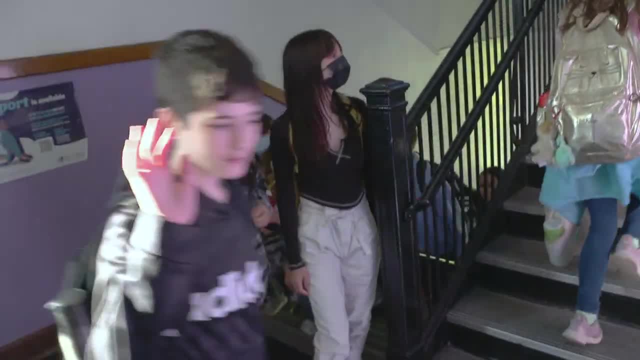 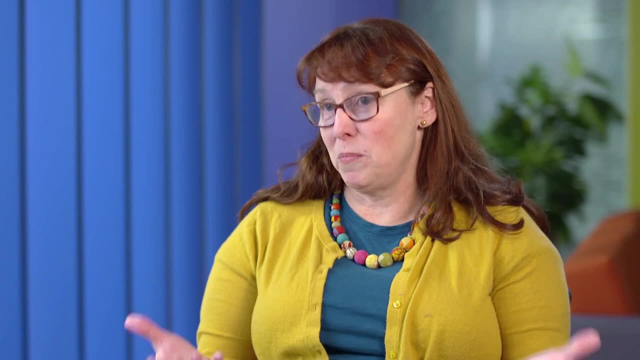 is it important to me to be good at math? And hopefully that answer is yes, because for your future it is good to be good at math. Life is problem solving. I would say the best definition of a good problem solver is someone who knows what to do. 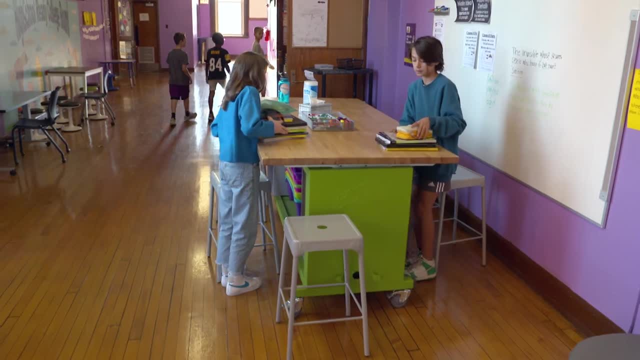 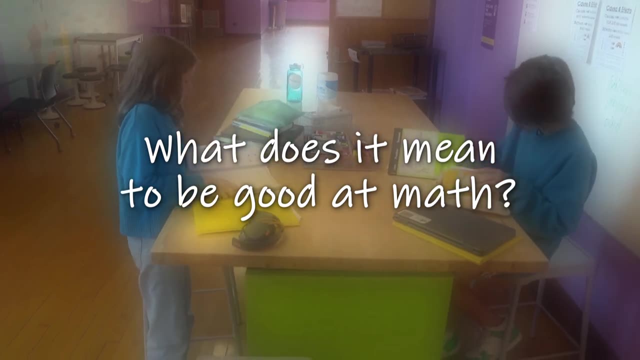 when they don't know what to do, And that's what we want kids to be able to think through and mess around with, and learn as they learn math. It means to be good at math, that you know a bunch of different strategies to get to the answers. It means to be good at math that you know a bunch of different strategies to get to the answers. It means to be good at math that you know a bunch of different strategies to get to the answers And even though, like your equation might be wrong. 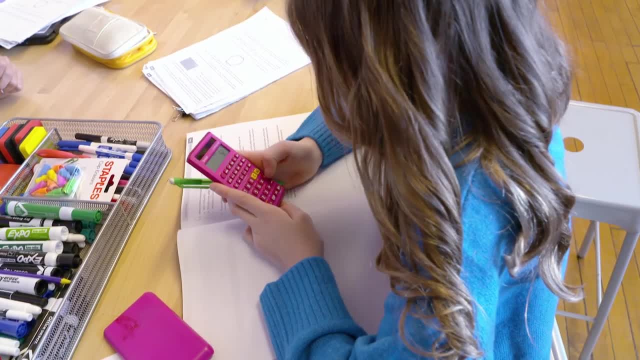 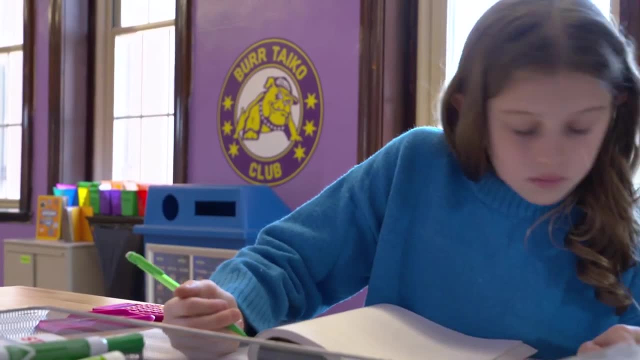 you have different ways to get to that answer too. There's a lot of beauty in equation because there's so many ways to get the answer and so many different strategies And that feeling at the end of where you finally solve it is really cool. 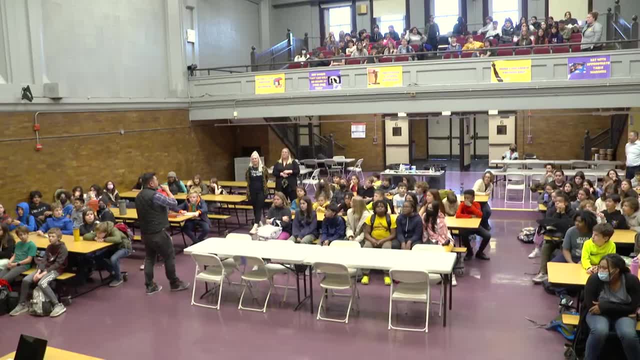 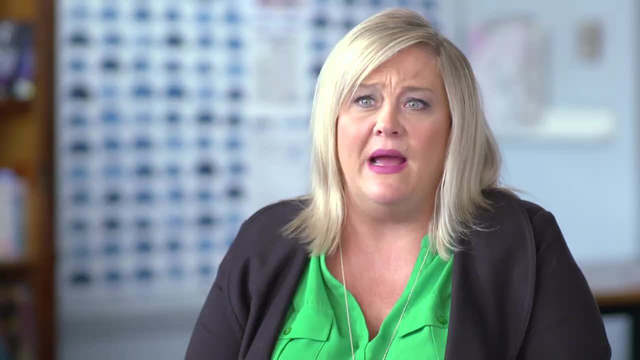 The history of math here at Burr is for the past 10 years. our reading scores were significantly higher than our math scores, So when I came in as the principal I had to say why. Why is this happening And what can we do to support. Because if they're able to meet or exceed standards in reading, why can't kids do it in math? We really had to look at the curriculum, And so that was the first thing in changing our curriculum and making sure that we had a really high quality. 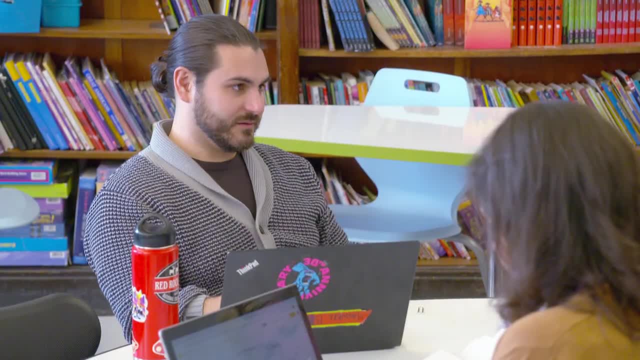 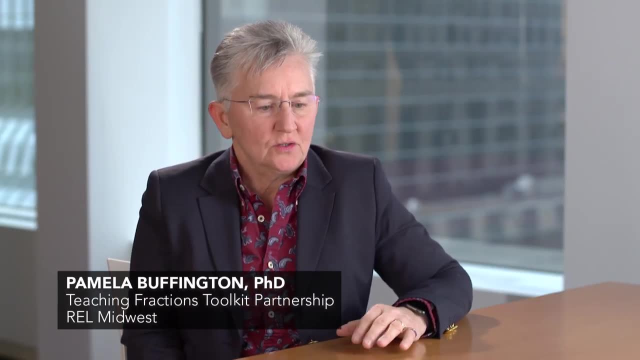 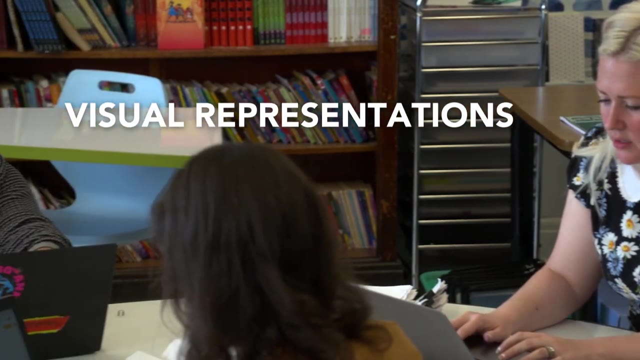 rigorous, research-based curriculum. And then it was: how do we develop our teachers around delivering this curriculum? Well, there are a number of evidence-based practices that contribute to and support student engagement in math. Three of them include and to use visual representations. 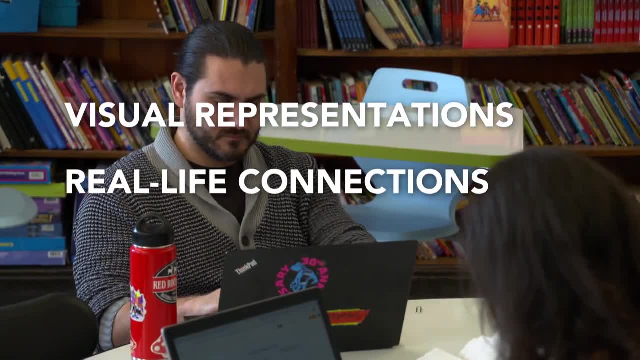 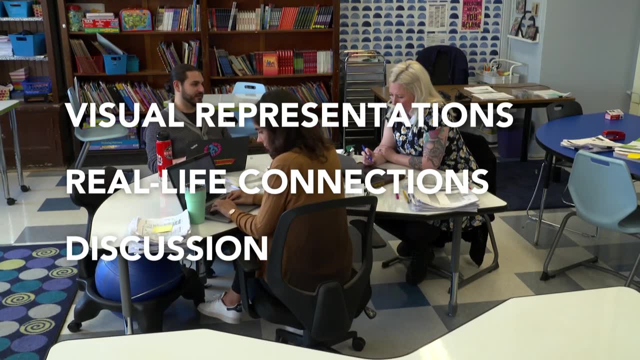 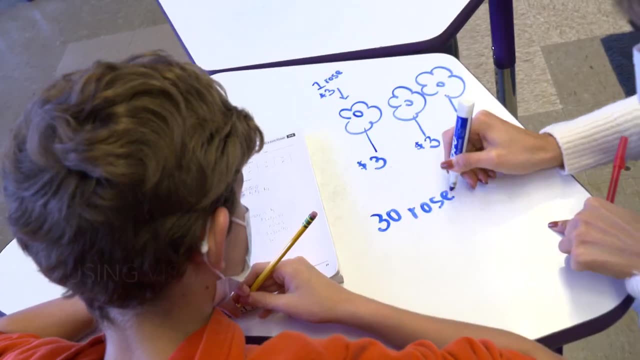 A second one is incorporating real-life problems with connections to student experiences. And a third, really important one is providing opportunities for students to have mathematical discussions with peers as well as educators in the room- The way that I would best describe the style of teaching. 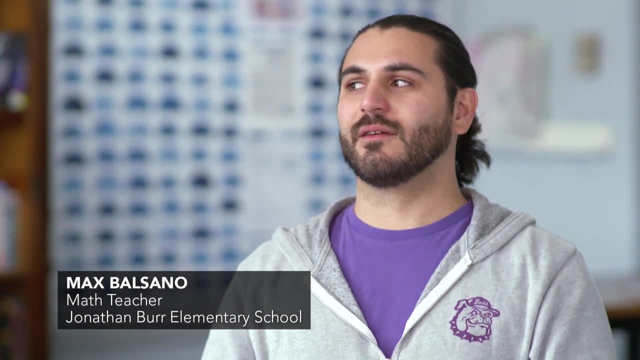 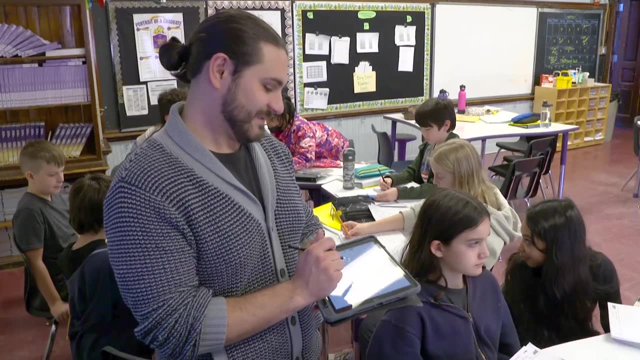 for the Burr Middle School math team is that it's really driven by flexibility. We know that kids are coming to us with a wide range of ability levels and day-to-day changes in terms of what they're bringing into class with them, And we know that we want to be able to meet them. 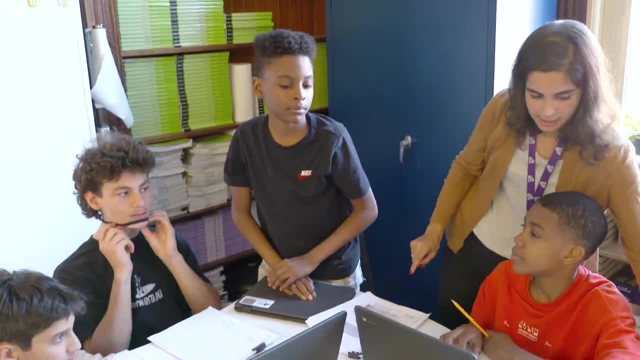 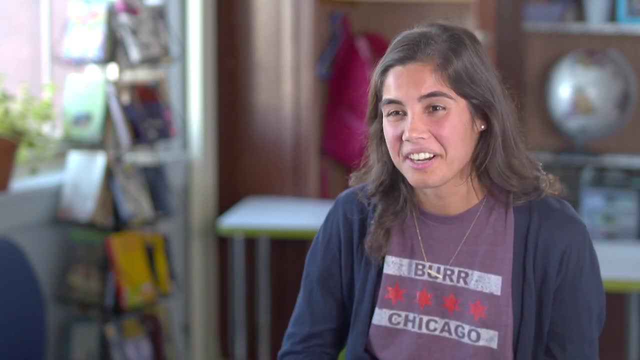 where they are. Our teaching style is very- how can I describe it? Our. it changes every day. I mean, we are just constantly learning from each other. We're just constantly adjusting our own practices to meet the needs of other students. 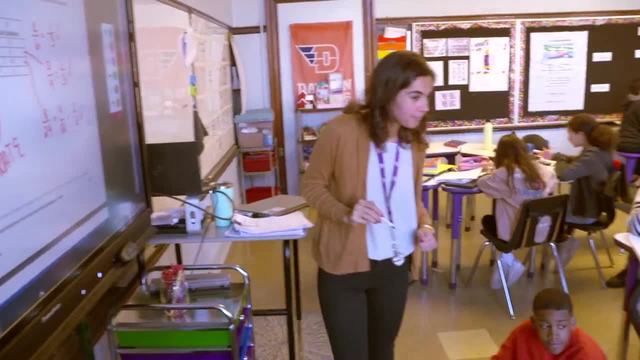 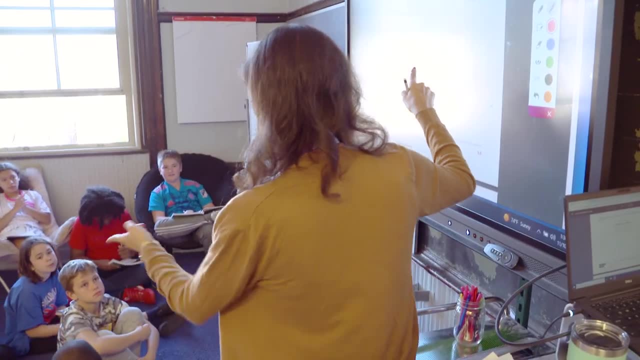 So there's not really one set structure in place. We kind of are just changing our roles and changing our daily practices to make sure that we're doing whatever we can to help the students. So for the students that are struggling, I think the most successful approach. 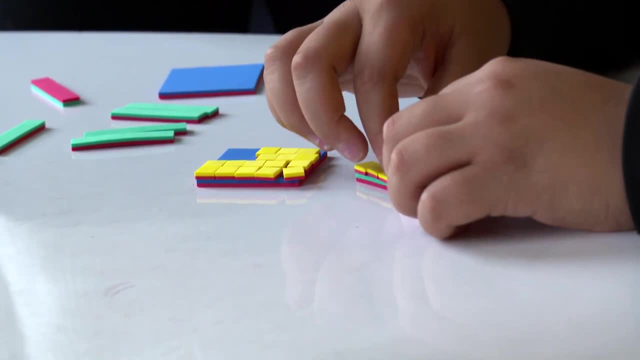 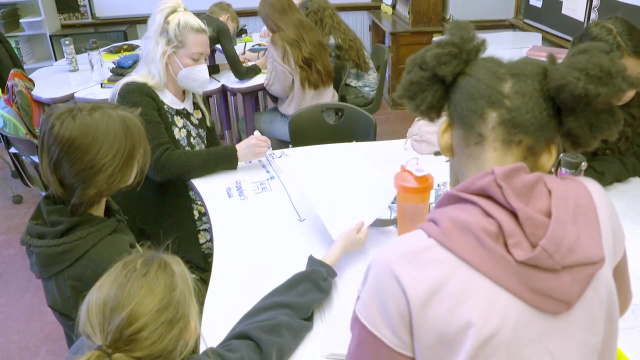 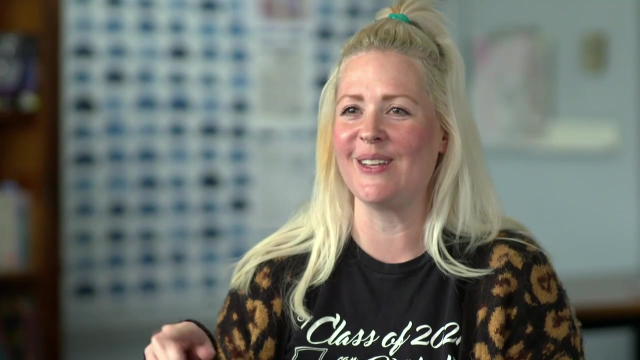 is either using a visual diagram or some hands-on manipulatives. I know for myself when I'm able to see the picture something, it becomes more concrete. I'm always telling students: draw out the problem. I am a terrible artist and you will see me drawing tons of stick figures. 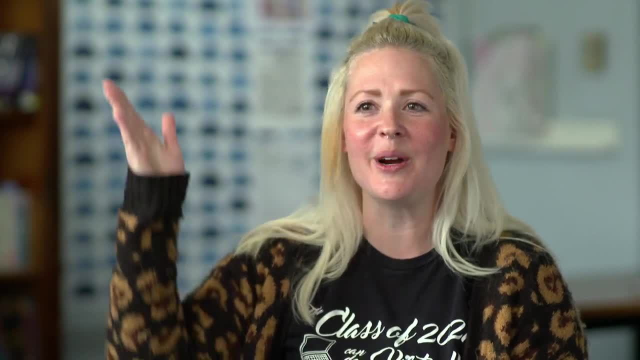 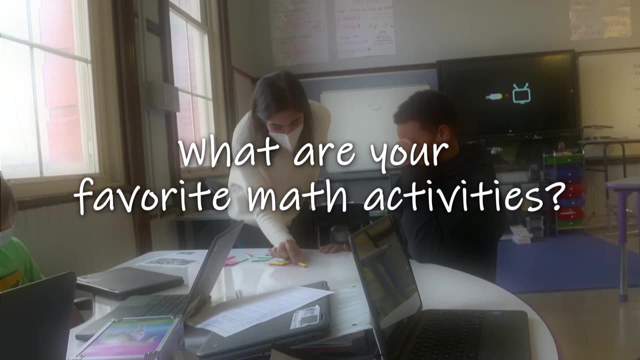 on that board, or like fishing birds on that board, to understand distance between below sea level and above sea level. There you go, Cool, So what can we call just this one piece? It's what fraction of the whole In the lower grades? 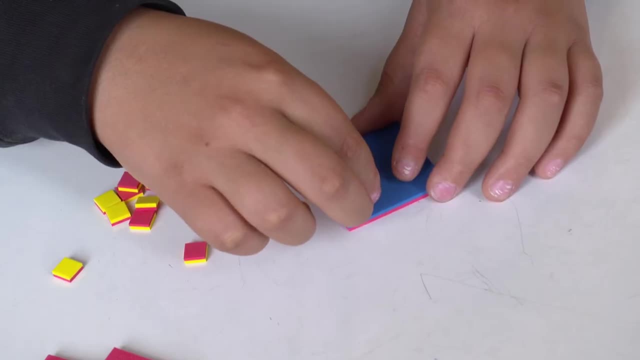 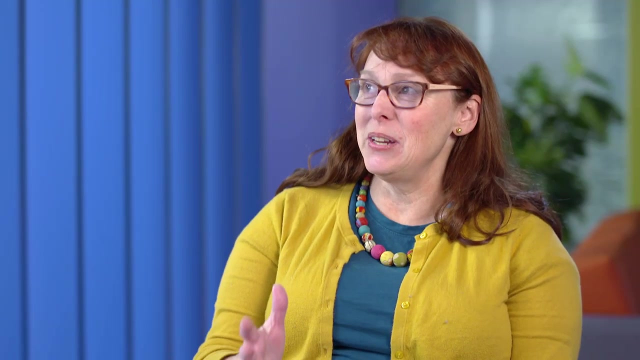 what made me like math more when they used to give us like blocks of a hundred cubes and you could actually count with the blocks and place the blocks on top of each other. So when students are in elementary school they often work a lot with pictorial representations. 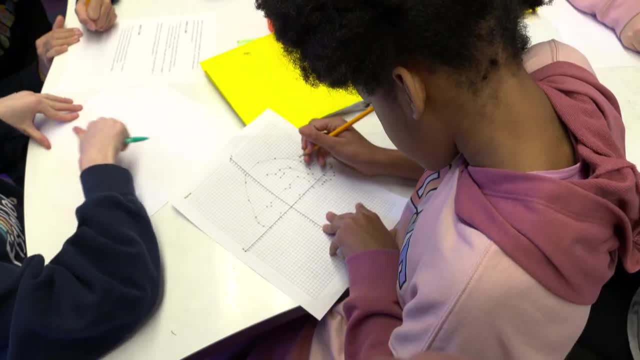 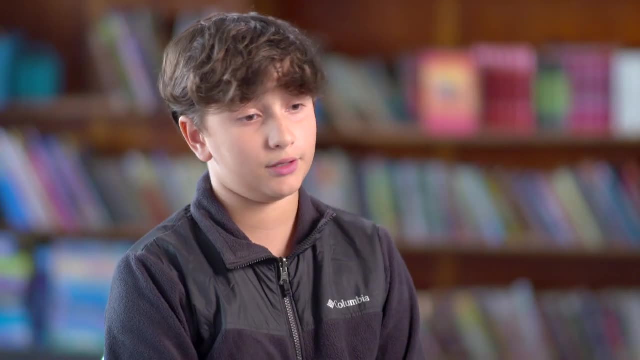 It's really important to continue that on through fractions as well, though, because being able to use a diagram or a picture just helps the student visualize it a lot more clearly. I had no idea what fractions were. I didn't think of them as like a part of something. 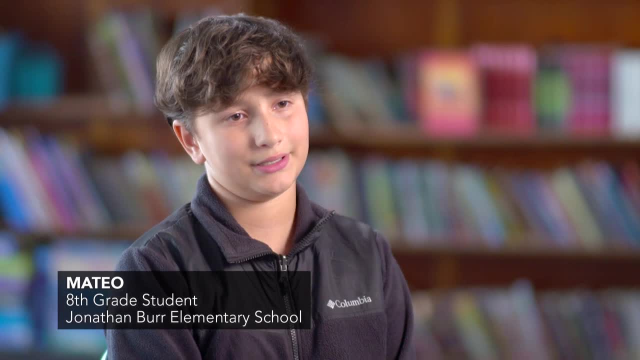 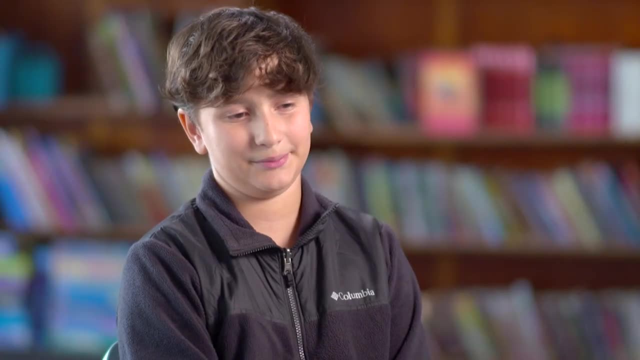 I just thought it was a number over another number And so I didn't really grasp the concept. She just showed me a different perspective, I think I think in pictures Someone says a car. I'll think of a car. Someone says four, eighths. 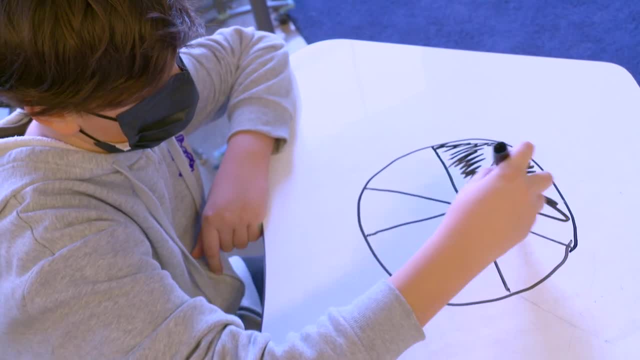 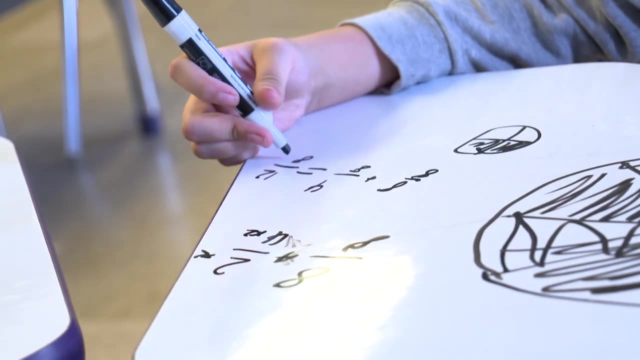 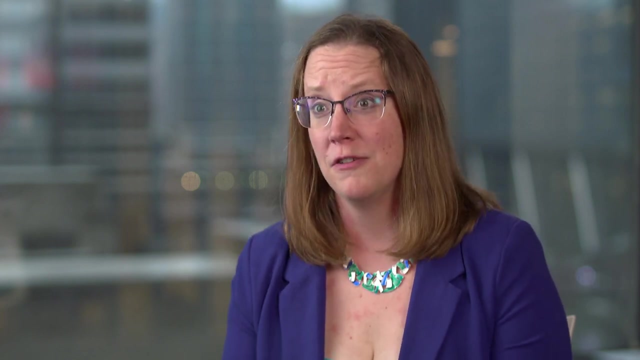 Then I'll think of a circle with four sides and four blinking. I think it works very well. I think their teaching is very productive and it helps students grow through their math. So CRA stands for Concrete Representational Abstract and it's an evidence-based framework. 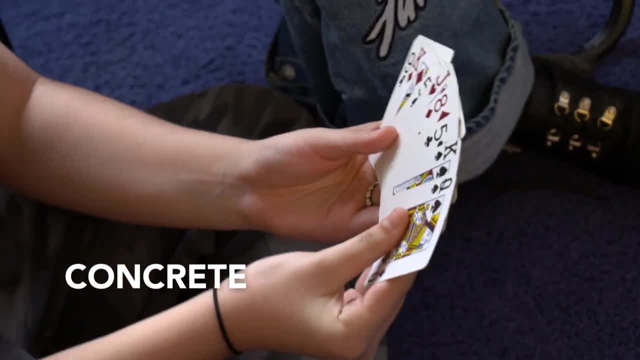 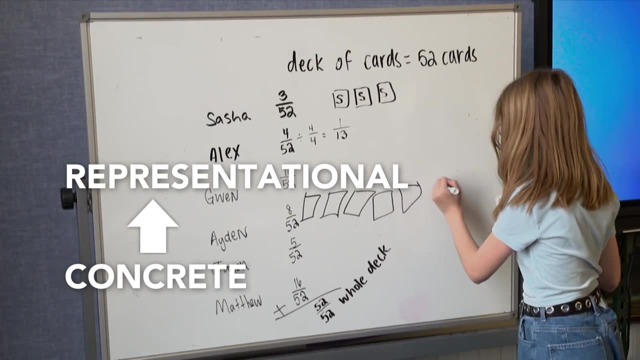 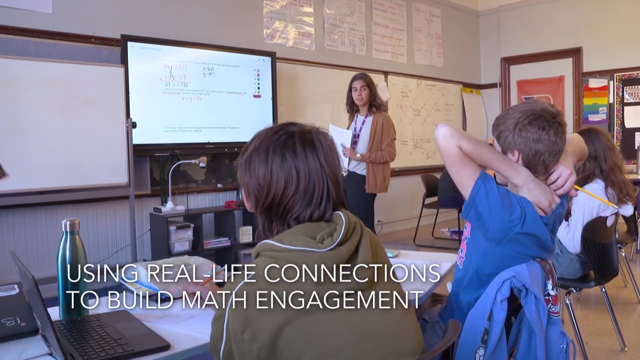 for how to sequence math instruction. You start with concrete experiences and then move to representational experiences, which is more about drawing and less about physical movement of objects, and then go to abstract, but focuses on mathematical symbols With fractions and other rational number concepts. 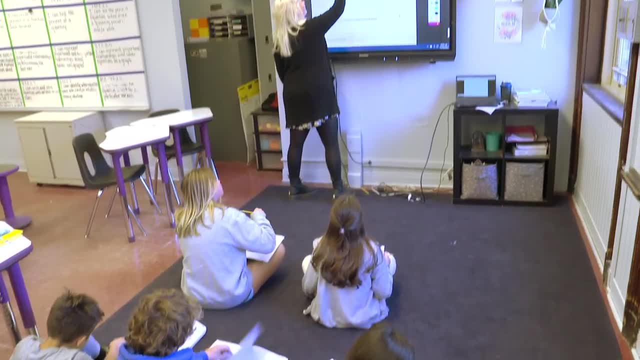 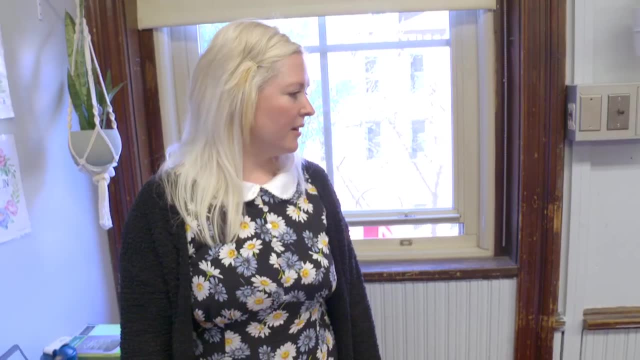 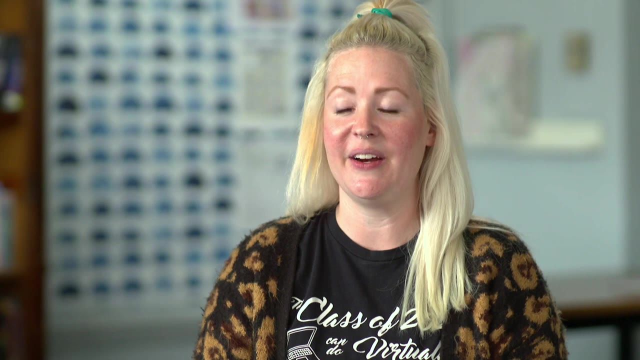 is they're very abstract And if we can connect students to real life applications and problems, it gives them a chance to dig deeper to see the connections and then the numbers have meaning. I will tell you, coming back last year after the pandemic. 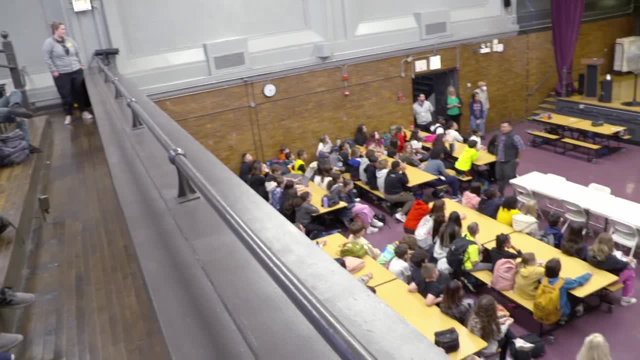 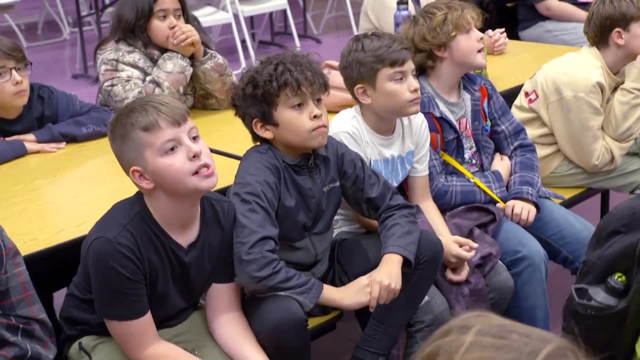 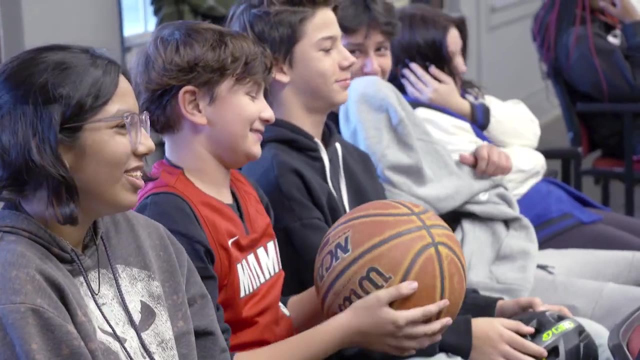 middle schoolers were a mess like social emotionally. We've really been working on addressing those social emotional needs before really diving deep into learning. The best way to get kids engaged in learning is really to get to know the kids first, because when 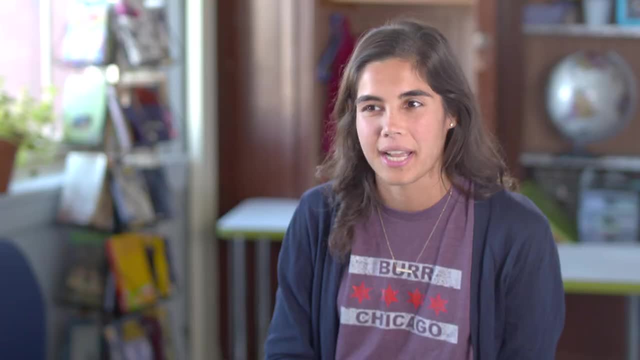 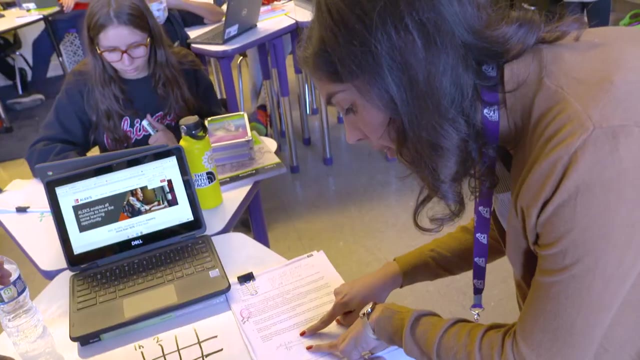 you have that relationship built with them and you're able to kind of relate to them and communicate with them, then it makes the material that much easier. So do you want video games to be the same or homework to be the same? It was a problem where it was a ratio of 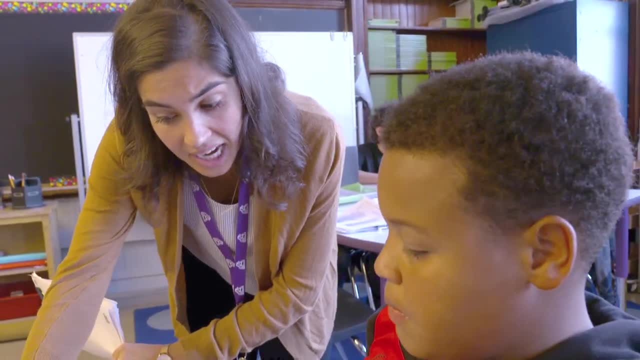 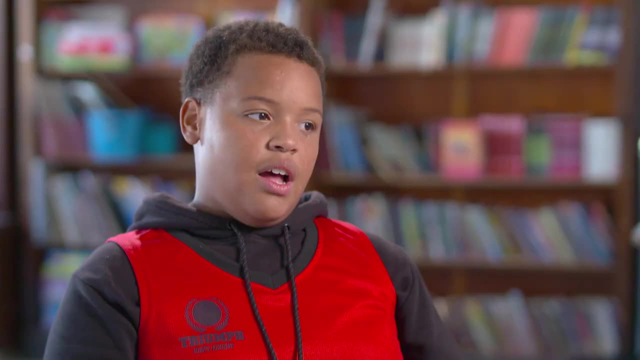 homework to video games and so say like: would I rather be John 10 hours to 5 hours of video games, or would I rather be Lucas to 10 hours to 6 hours of video games? I like it because I like adding and going up and 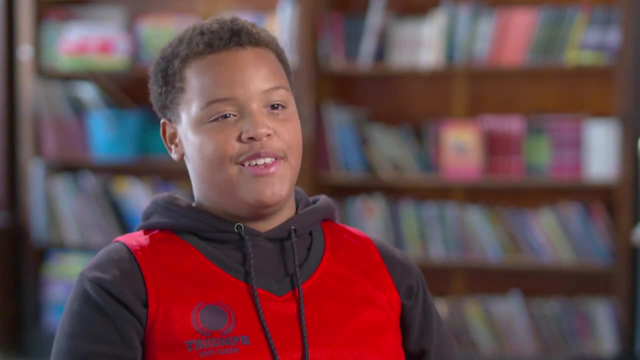 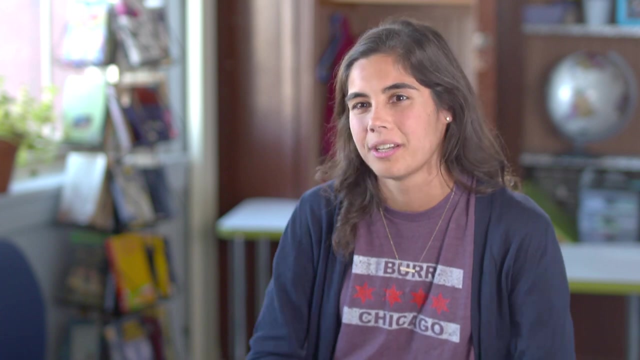 then doing the ratio and seeing who has more video game time. We try to always relate it back to why do I need to know this in the real world, because that's everyone's question. What is important? What is the importance of algebra? and aside from 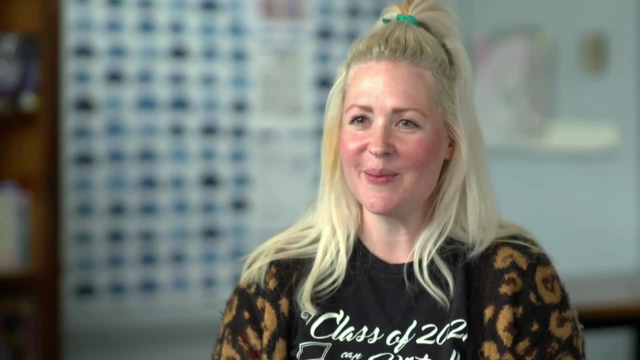 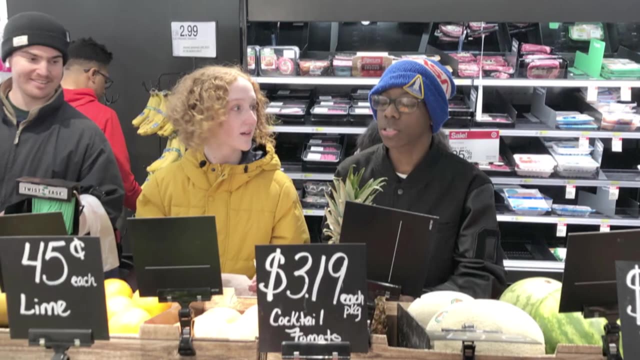 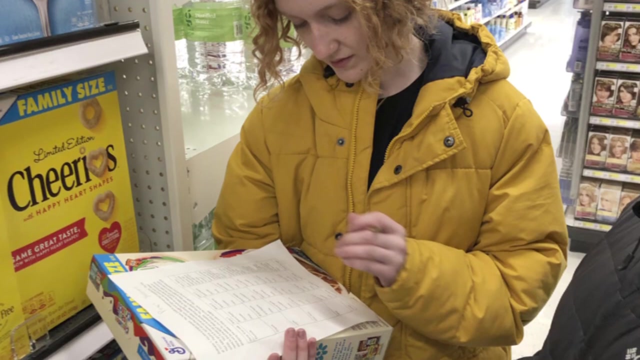 passing this test. why do I really even need this? We go on a field trip to Target and Jewel and students calculate discounts. So during our percents unit, one of the big skills that we need to know in sixth grade and seventh grade is how to calculate discount. 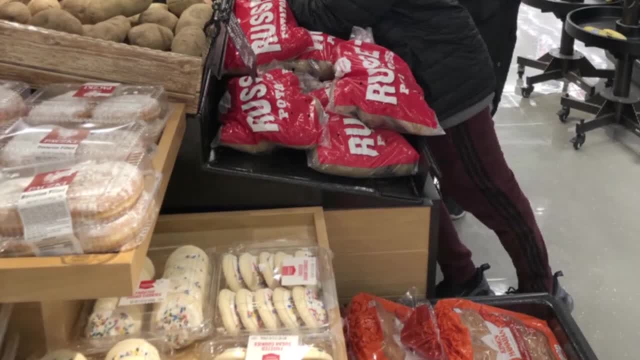 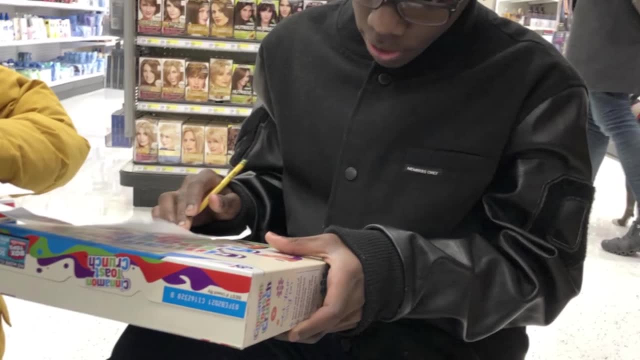 I take them out into the real world and I go: okay, like we're at a store, let's find things that are on sale, Let's look at the original price, Let's get the discount and let's calculate what we're going to pay for it. 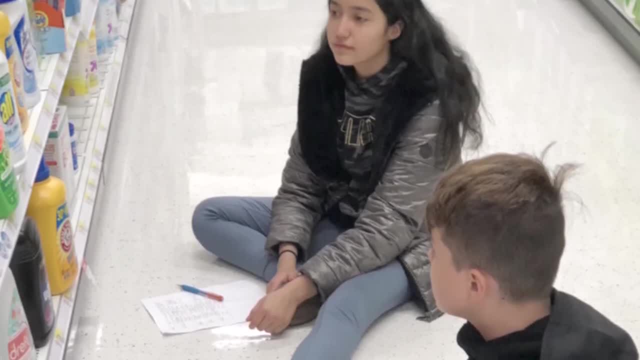 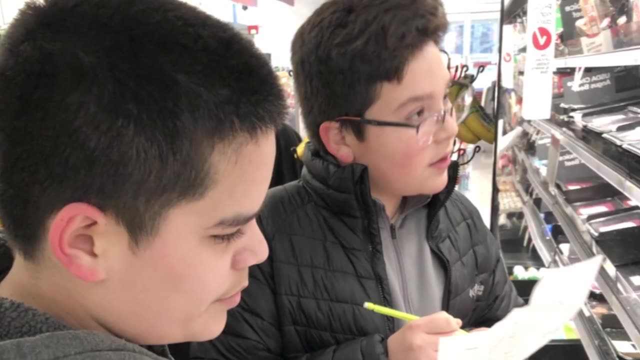 And I gave them a situation. You're a college student. You don't have a lot of money. You are on a budget that is this amount and you need to buy this, this, this and this. Go, try and find the best deals that you can find. 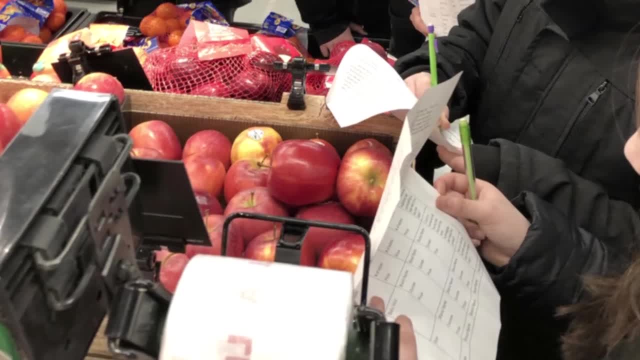 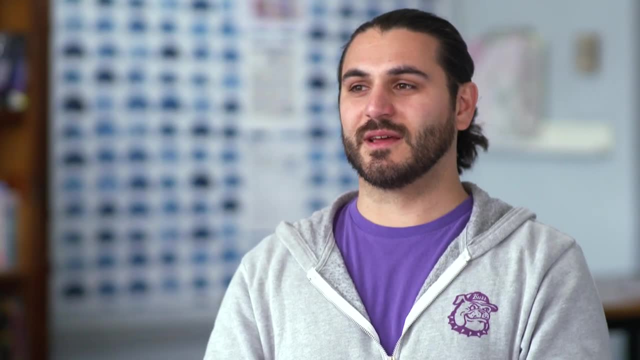 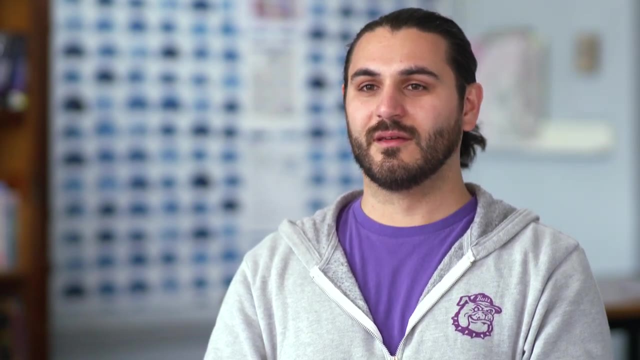 I felt like it was a really meaningful and exciting experience for the students and the students talked about it all year. I think it's important to mention to students that math is super important, but the skills that you need to work on and attempt math that will. 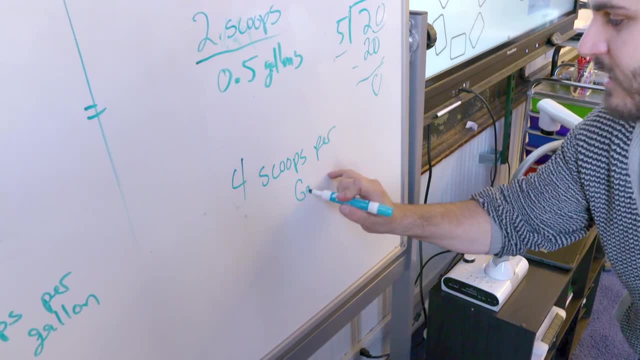 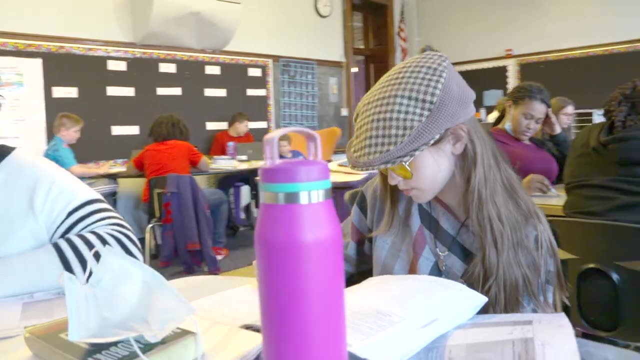 apply to your everyday life are equally as important. So, even if we're not practicing math, to be able to attain and do math at a college level, we want to see you be able to apply basic problem solving skills. We want to see you to be able to work systematically. 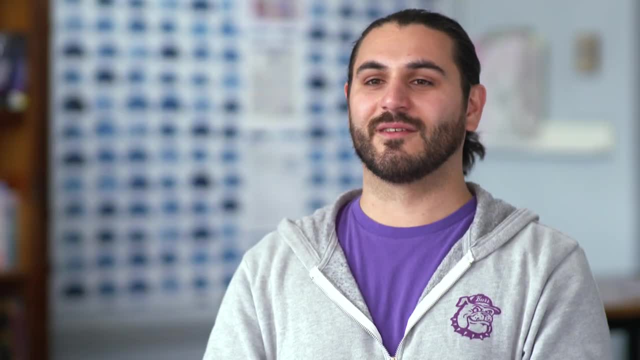 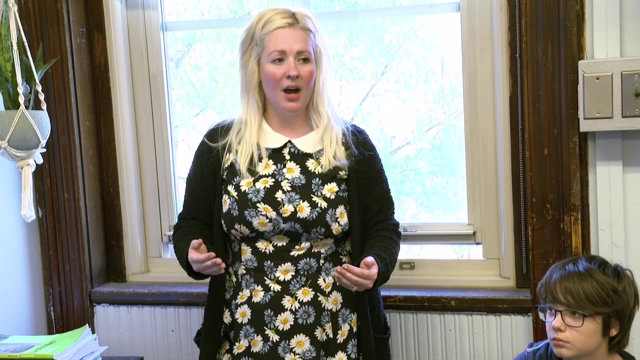 and attend to precise work. If that is in math, that's great, And if it's in your hobby, that's awesome as well. I think also just the math teachers being really excited about math and kind of being animated in the classroom and being like: hey, I just used this. 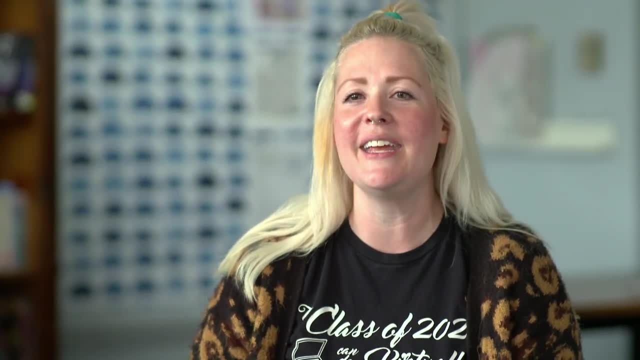 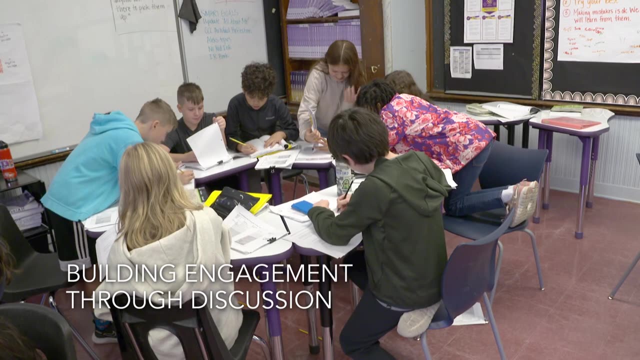 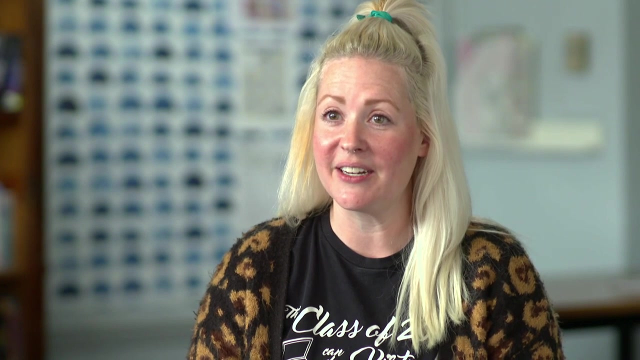 the other day I was trying to find, you know, a couch cover and I calculated surface area. They've got a lot of hormones, They're growing and changing And so I feel like, especially in math, in a subject where you're trying to figure out how to 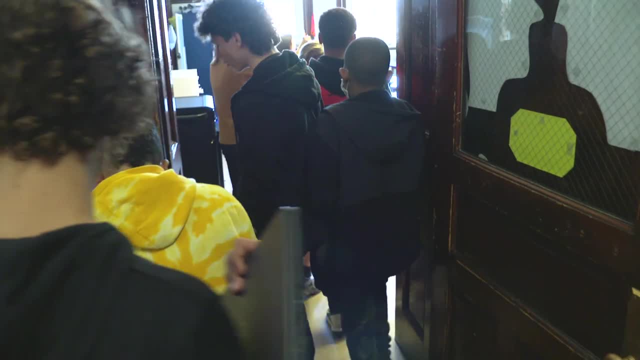 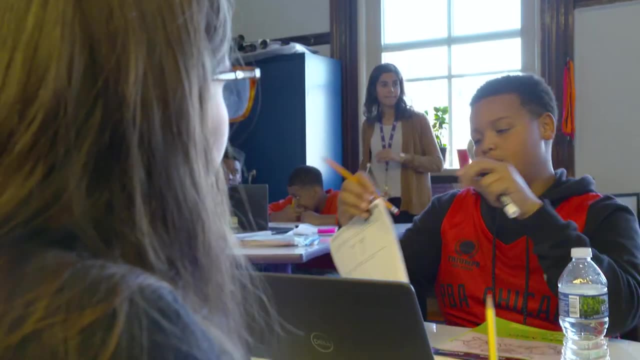 work with a peer. students usually don't come into the class super enthusiastic. Being able to give them that time where they can work with a peer or work with a group really benefits them. Communication is a big piece of math that is often overlooked. 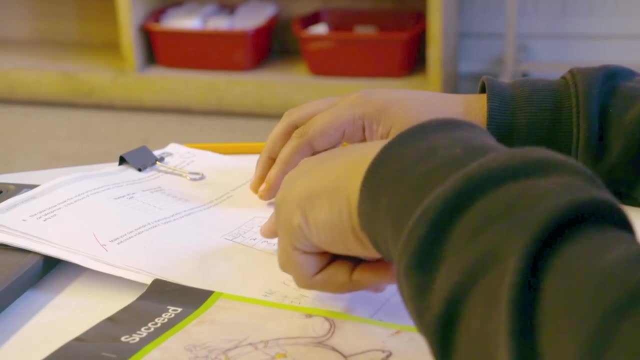 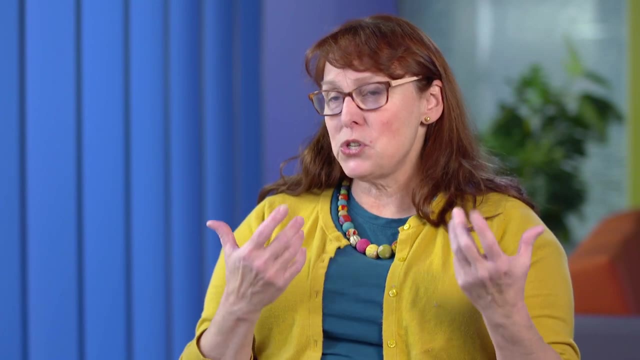 We tend to think of speaking and writing happening in an English class or in a social studies class, but maybe less so in a math class. But to me it's very critical there because as students talk about the math, either back and forth with a teacher or with a teacher, it's a 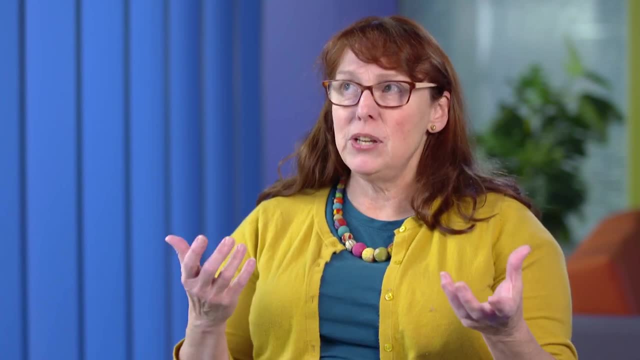 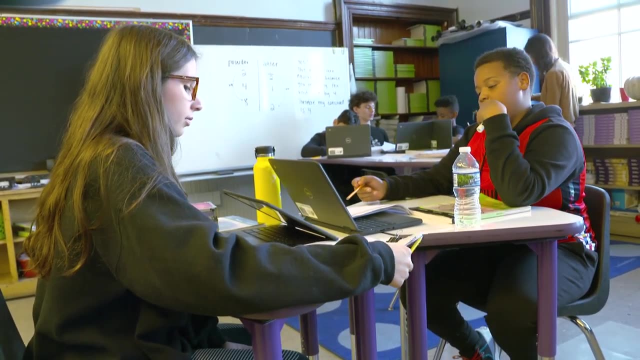 great way to communicate with a teacher or with one another, which is great too. they have a chance to kind of get their thinking out there, And often, as students talk about their own thinking, they can revise it. they can revamp it. 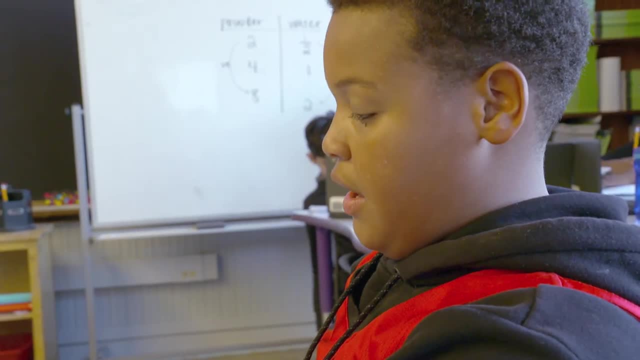 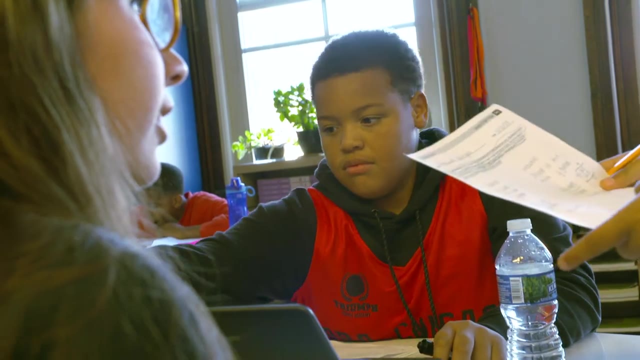 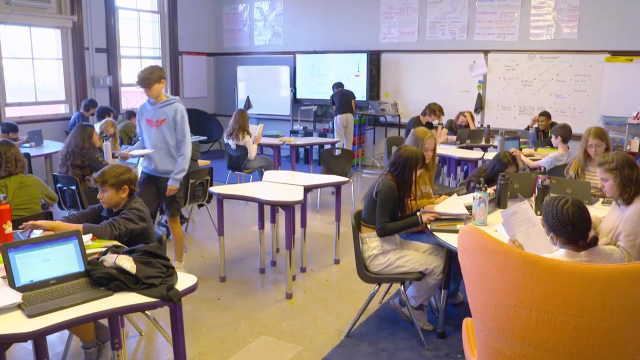 If you think about mathematical practices, habits of mind that we want students to learn in mathematics, part of that is being able to create arguments and critique those of others. So communication is a big part of that. Can I formulate my thoughts? Can I also look at someone else's argument and say: 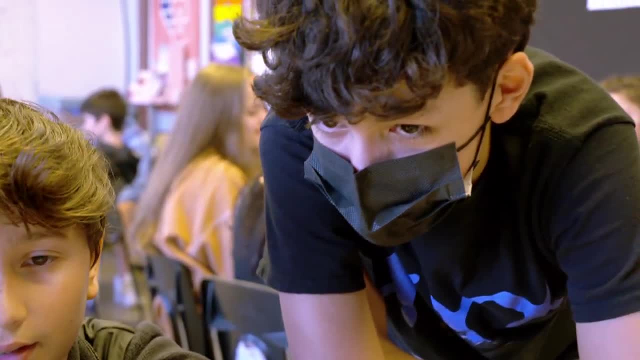 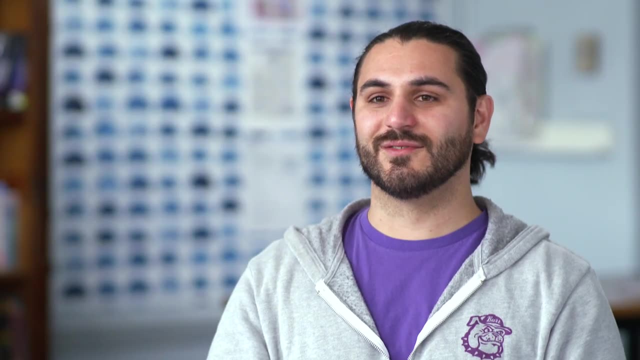 hmm, does that make sense? Does that not make sense? Where does it break down? Or is there maybe something in their argument that makes me think of something else? Our goal daily is that students are having opportunities to talk about math. When I'm teaching a lesson, I want to speak as 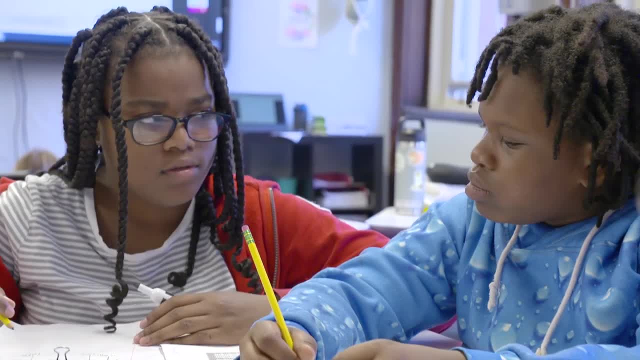 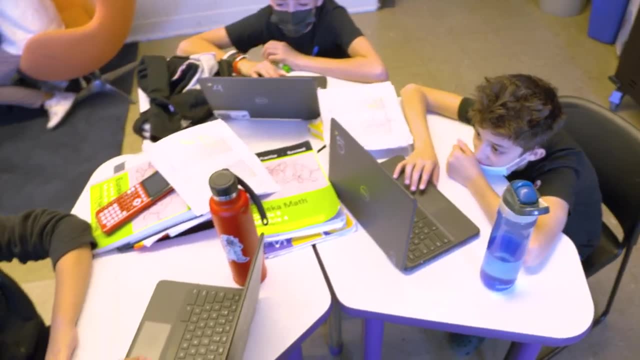 little as possible to give as much space for student voice as possible. We do whole group instruction where the kids work on a on-grade level task in all mixed groupings So they're able to communicate with each other and say OK, even though I might not have access to. 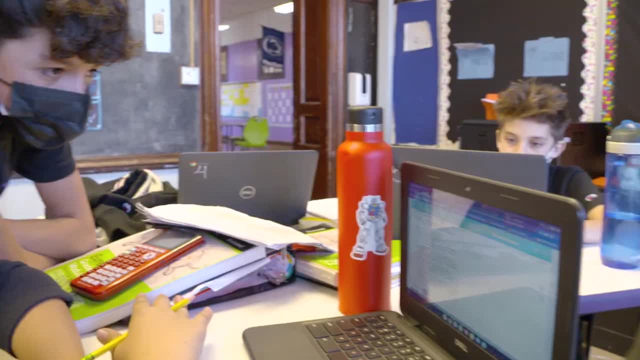 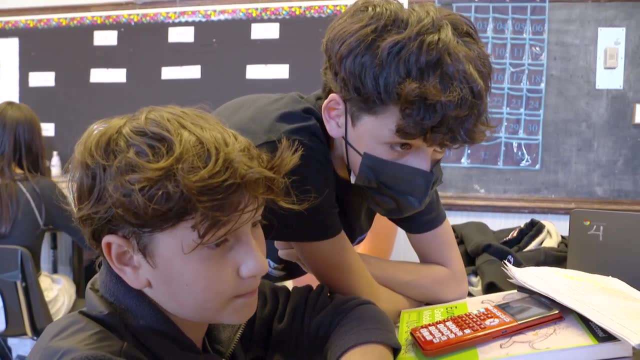 this material I can communicate with the rest of students in my group so that we all can reach a common goal. Sometimes the most knowledgeable person in the group is not necessarily the most knowledgeable person about math in the room, but it gives them the opportunity to take on that leadership. 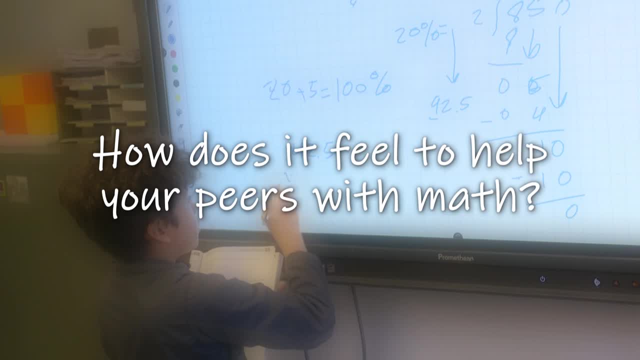 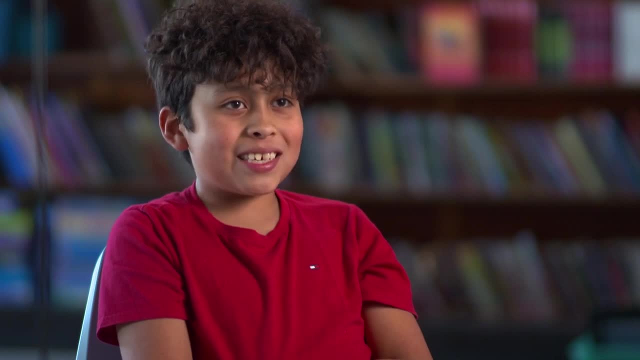 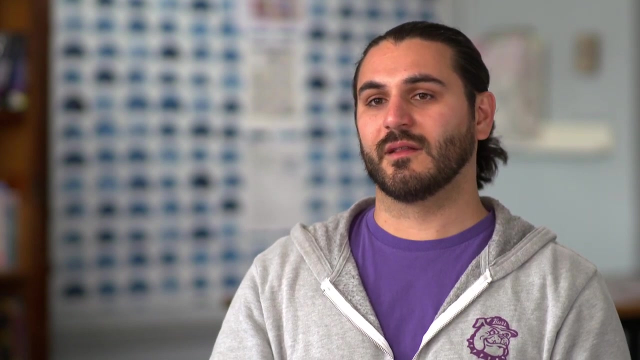 role and really talk about their math thinking, which is great. It feels good because they come to me asking help and it's just cool. We find that getting input from your peers is sometimes more valuable than getting that same input from a teacher, So we want to make sure that they're having those. 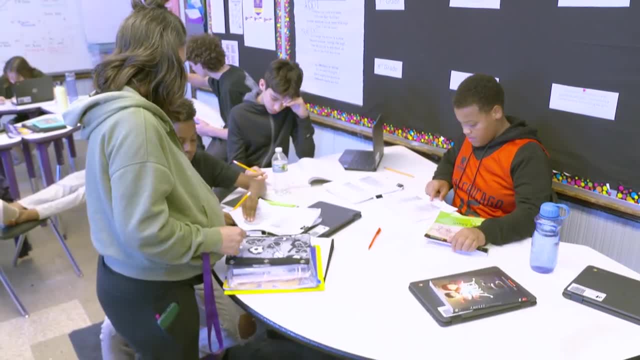 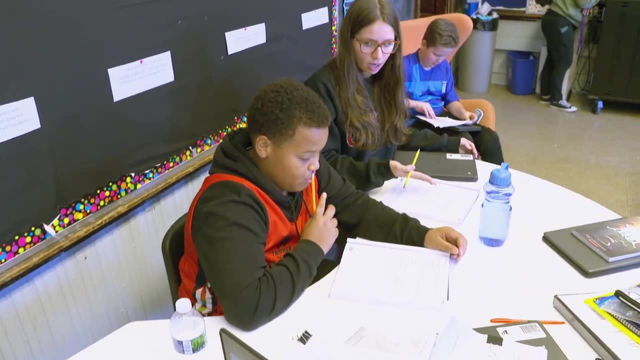 moments of, like, intelligible discussions with each other about math topics. I love helping my peers with math because, like it just makes me feel like a good person and it makes me feel like I just I'm really there to, like I'm really a purpose and I really did something. 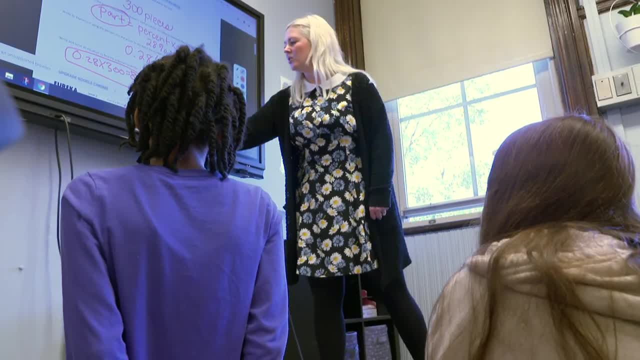 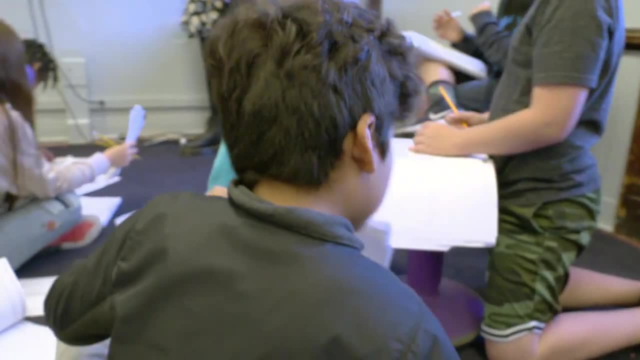 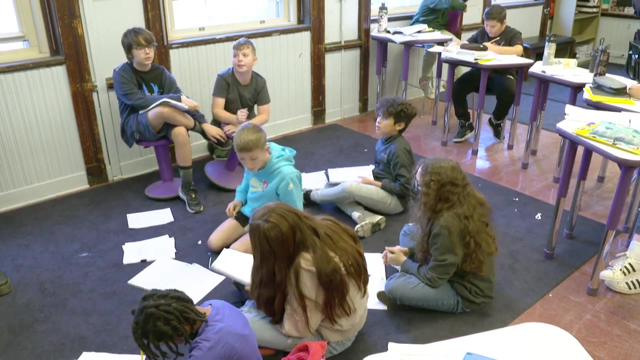 I usually present a problem and then I give students three to four minutes to talk to each other to try and solve that problem. So I don't ever give them the steps right away. So they have to productively struggle and some of them do struggle and some of them are very 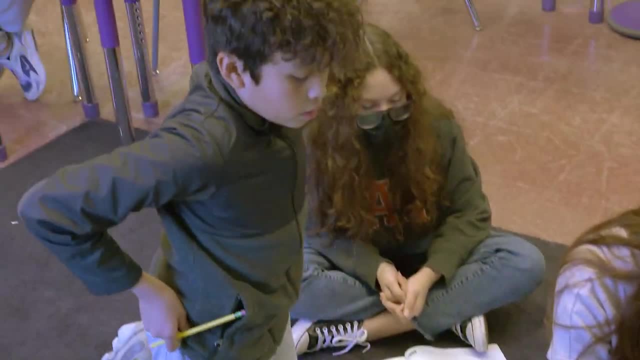 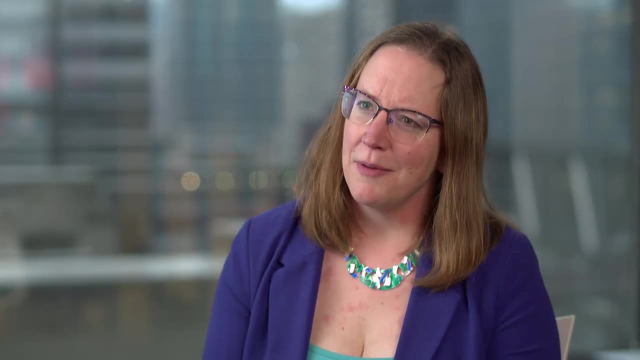 productive with it. I want to put them together on that carpet so they can kind of talk through it themselves. In classrooms we see a lot of the explanation happening when kids are finished, or you know, the high flyers in the classroom do all the talking. 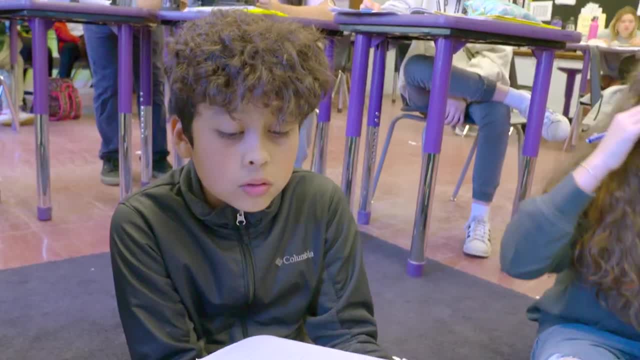 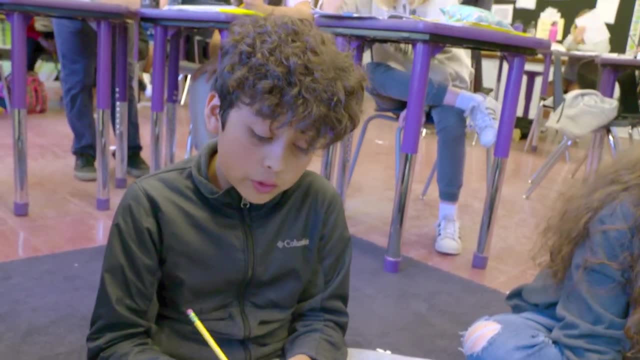 So integrating more opportunities for kids to talk to each other and work out their thinking together really gives them a chance to see when they're making progress and can build their math identity. Ms D's style is like she always gives the kids an opportunity to try to solve it themselves before. 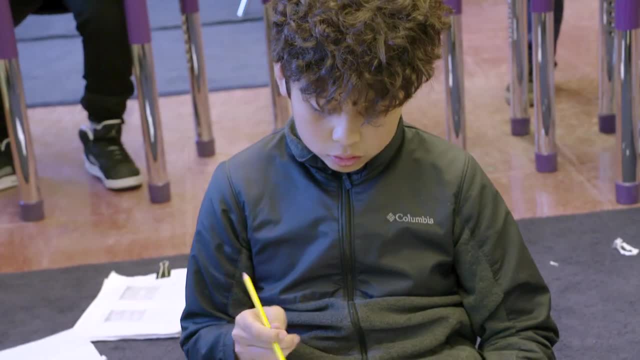 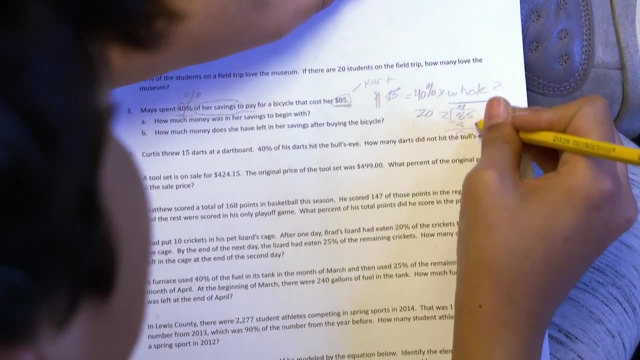 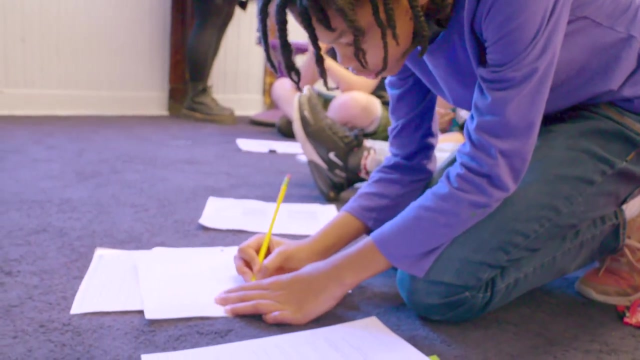 helping because, like you're never going to learn, it's just somebody helps you all the time. So she tries to let the kids work with themselves, like together in a group, and it helps me a lot to acknowledge what they're saying. Students do better when they have a chance to talk. 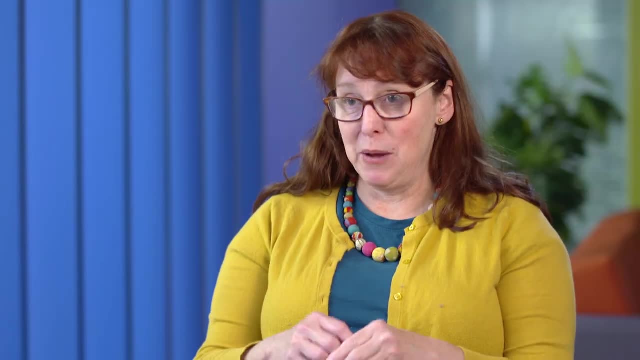 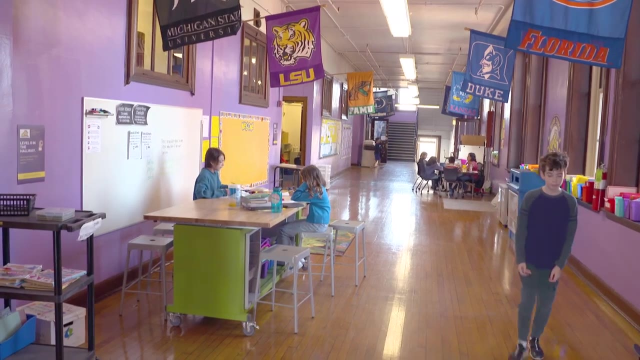 about the math, and math isn't just something that happens on paper that the teacher looks at. So if they have a chance to kind of mess around with the math, and math doesn't become just a search for a correct answer. it becomes more of something that you interact with and possibly 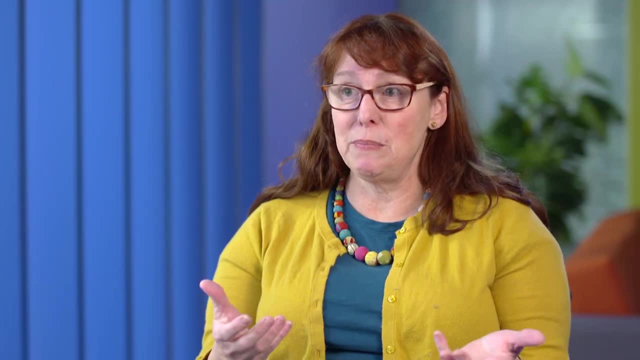 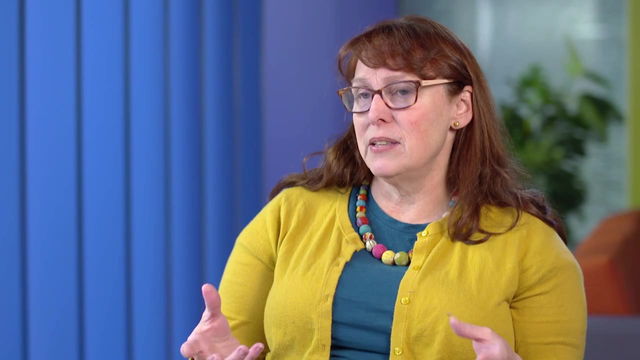 get to a solution. possibly you don't get to a solution. It's always interesting. maybe you're working on a problem where there's multiple solutions or multiple ways to get to a solution. It helps kids see what they're doing. It helps kids see the flexibility of math. 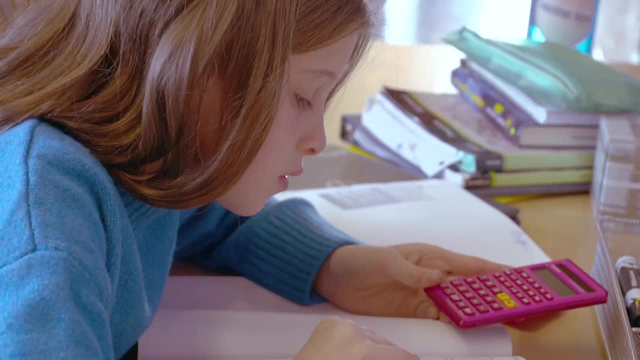 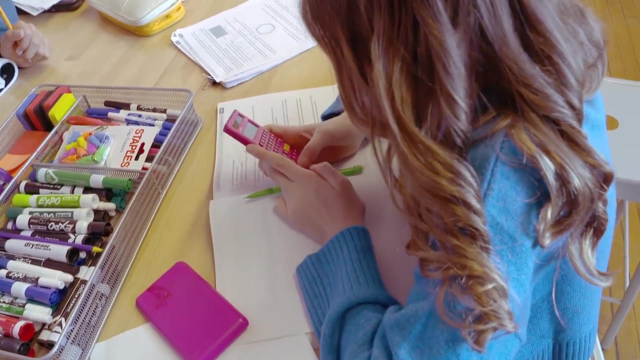 That sometimes you just can't figure it out and it can be like really hard, Tricky or like kind of like a dead end. sometimes I'll try different strategies until I feel like it's mostly right Giving kids things that they have to struggle with. 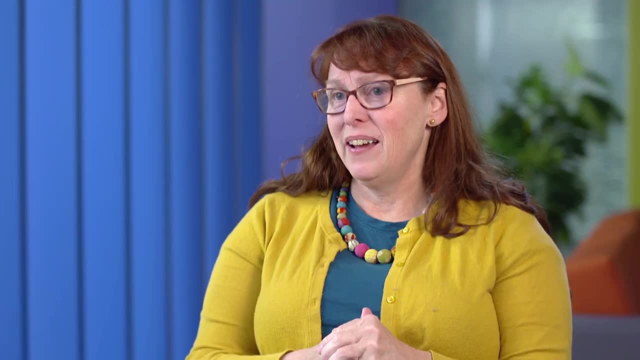 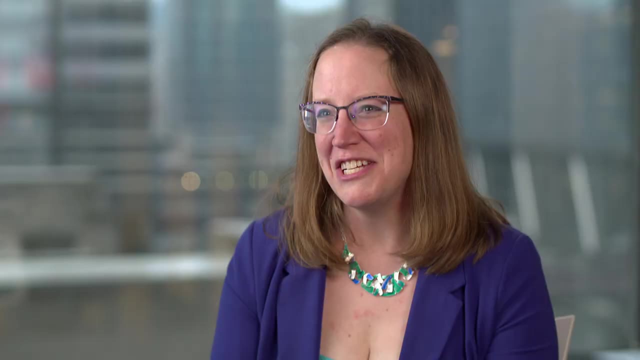 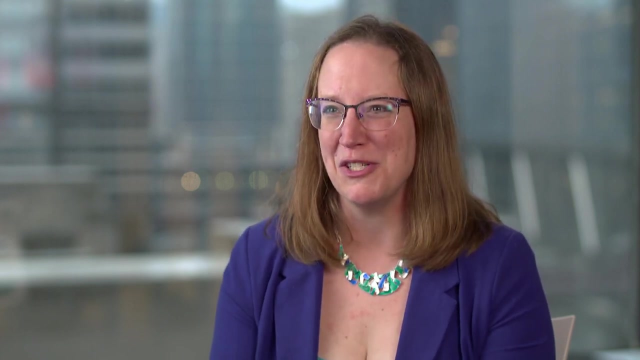 a little bit builds perseverance and problem solving, and that's something that is needed no matter what you decide to do. So computational thinking is a set of practices that computer scientists do as they engage in their work, and there's some key examples of those we really focus on. 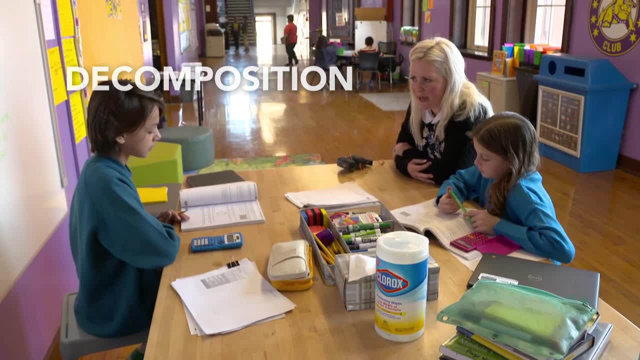 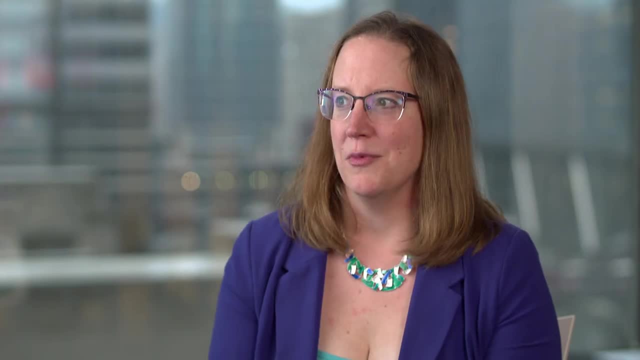 So one is decomposition, or breaking complex problems into smaller parts. Sometimes the equation isn't there and, like word problems, you have to figure out what the equation is. Another one is abstraction, or identifying the really important things to focus on and representing those to guide our thinking. 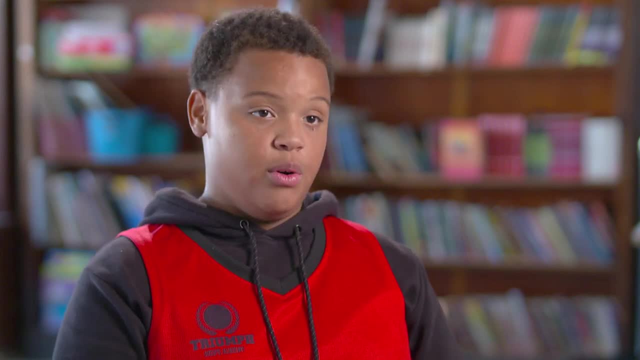 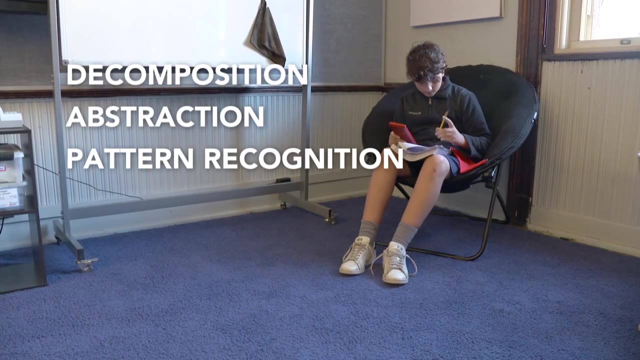 Underline like all the important things and then circle like the really important things. I'll just like cross out any unimportant words. We also think about pattern recognition. So what patterns do I see in this problem or among problems that I can move forward in my thinking? 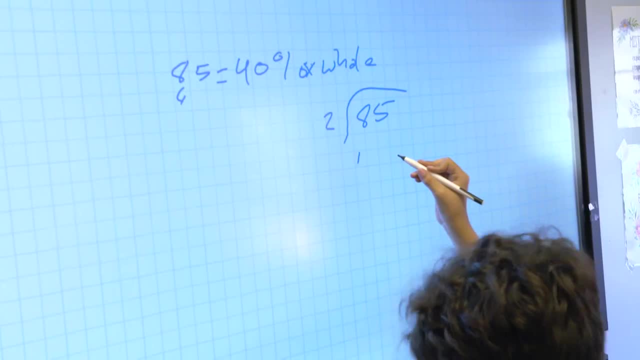 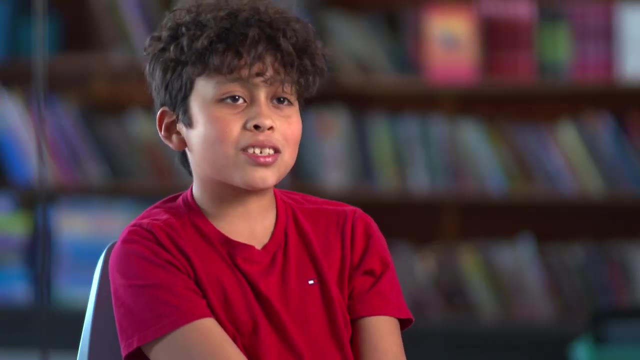 Algorithms are step by step instructions that we can develop and kind of carefully follow as we solve problems. If it's a division, I would divide next. If it's a multiplication, I would obviously multiply. If it's like fractions, maybe I would try to simplify. 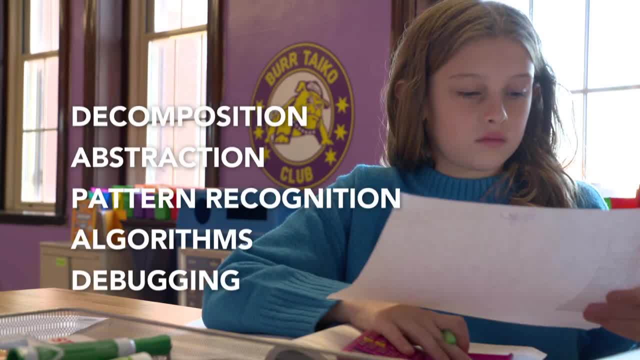 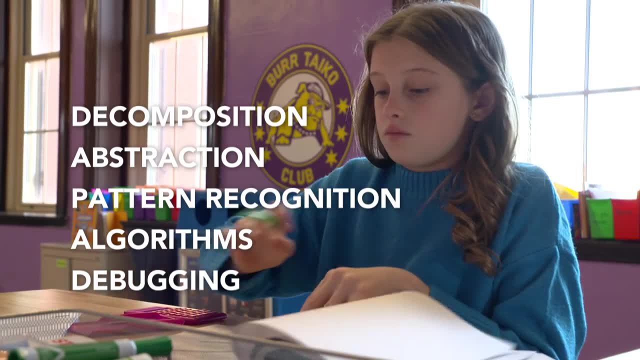 And there's debugging, which is a process of looking at your work when you make a mistake and really trying to hold up the things that you've done that are really good and fixing the small errors you make so you can move forward And if I can't, I will go through that process again. 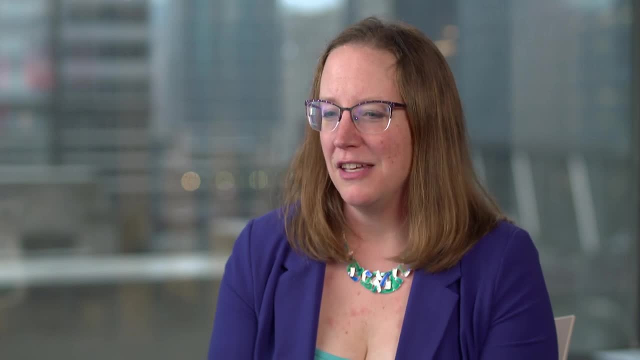 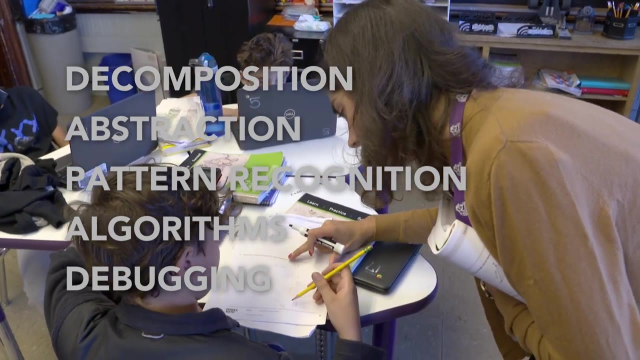 until I can get an equation and then I'll solve the equation. So computational thinking can increase engagement because it gives them a few words and a few concepts to really grab onto. Maybe I can try decomposing this problem. Maybe I should do some debugging and see where 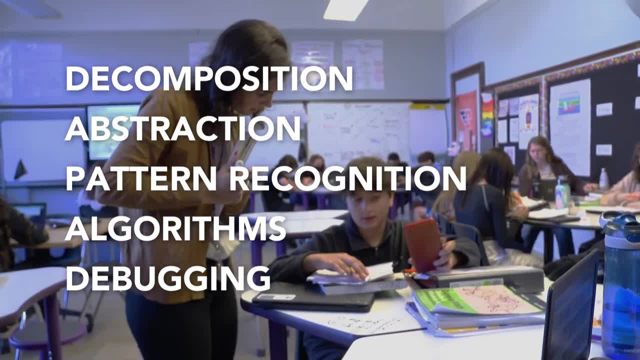 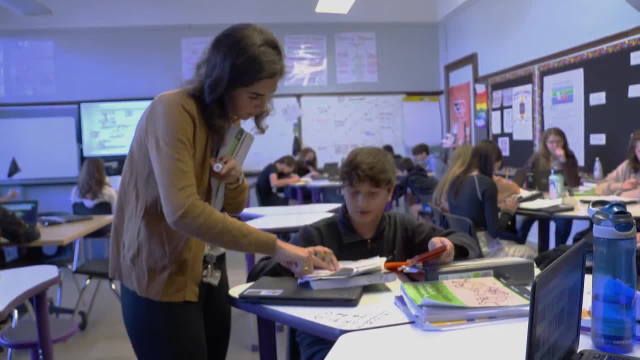 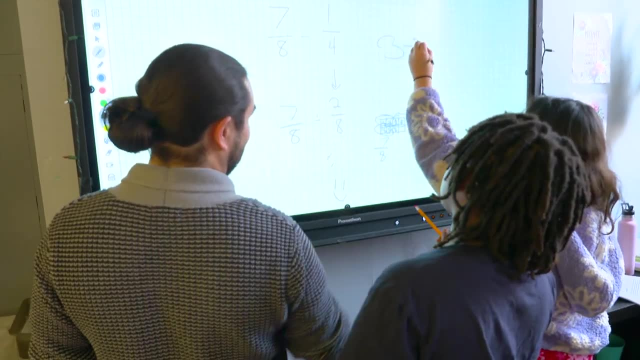 my mistakes are. So there's some really concrete strategies in there that gives kids tools to get into a problem and get past that And that gives them that initial hurdle of I'm not sure what to do next. Regional Educational Lab- Midwest. So we partner with educators and policy. 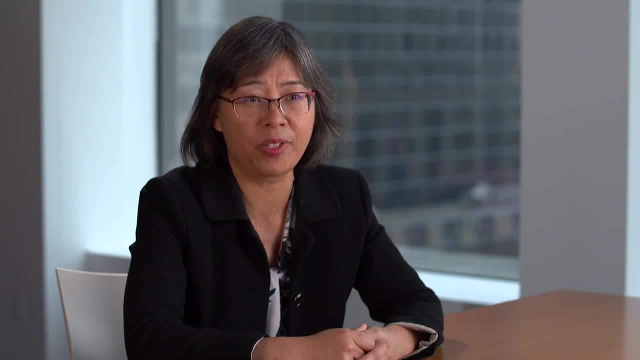 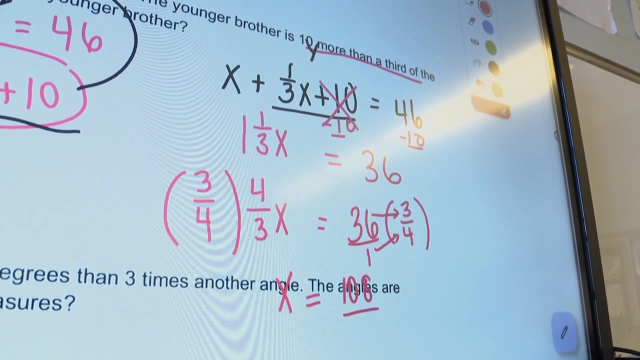 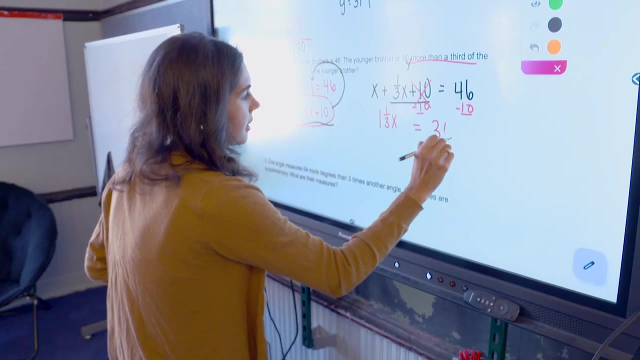 makers to support their use of data and research, with the ultimate goal of improving student outcomes. American students often like have difficulties with fractions related content, and this is well documented in literature. This difficulty is not confined to students as well, like teachers. there's plenty of research. 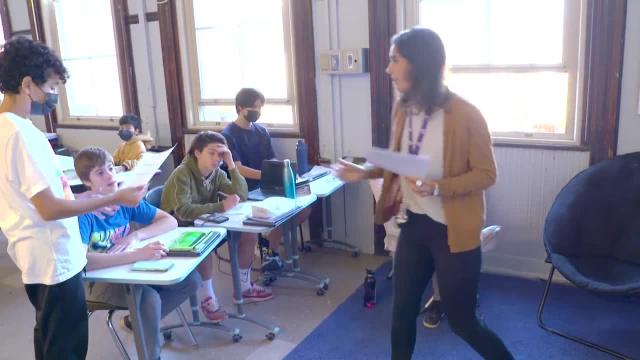 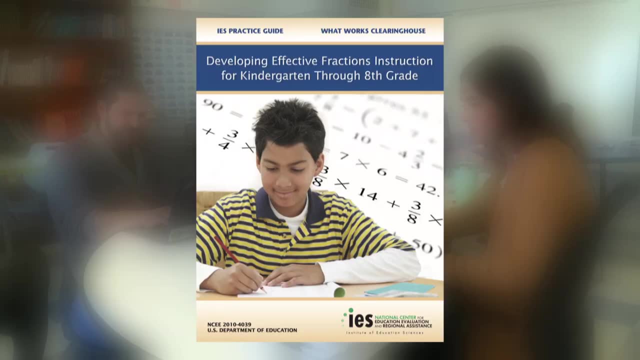 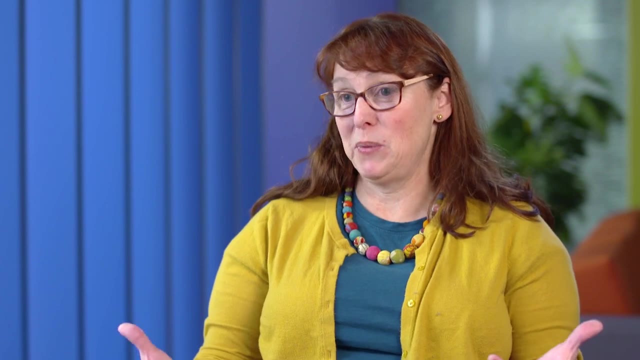 studies saying teachers often struggle with fractions related content as well, So they also need support on this. So the Teaching Fractions Toolkit: we focus on providing support for teachers. So the goal of the Teaching Fractions Toolkit is to take the evidence-based strategies. 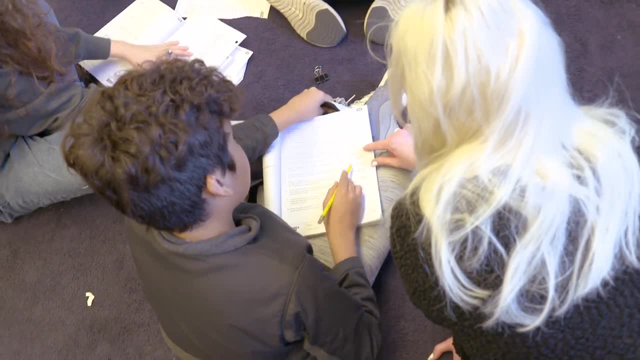 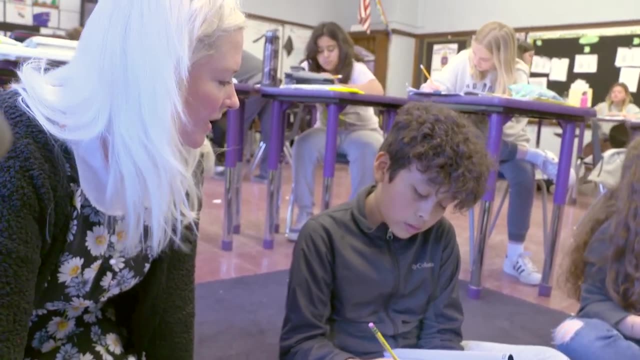 that we see in the What Works Clearinghouse Practice Guide and help teachers translate those into action. And that's what we're going to be doing in the classroom. Many teachers already do some of these strategies. The toolkit will help them use those strategies even. 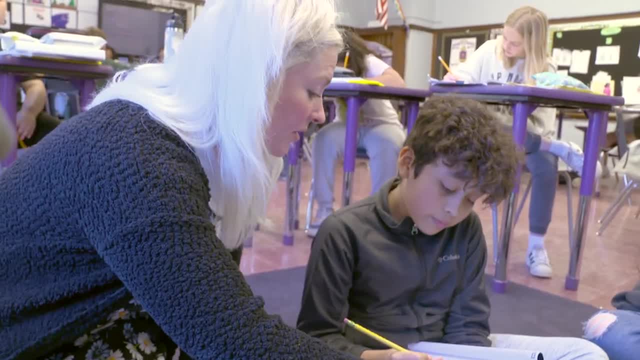 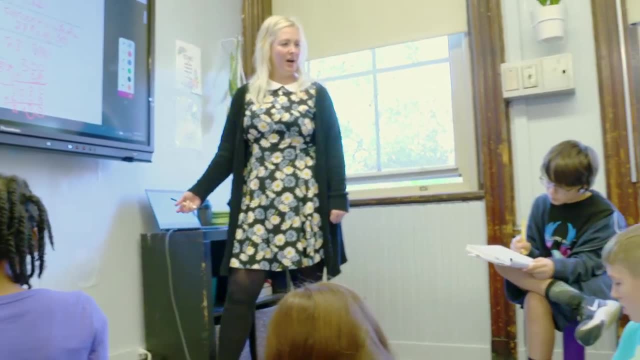 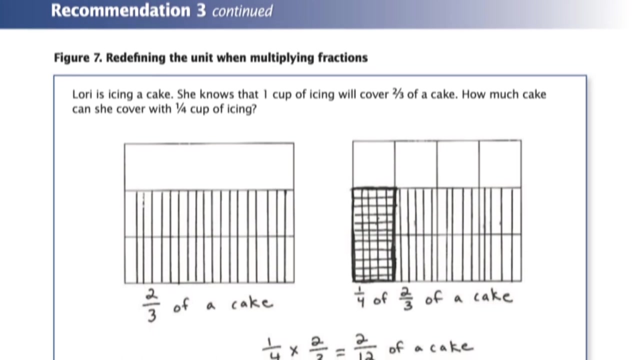 more effectively. It's going to give them prompts and questions and things they can use directly in the classroom, not only in teaching the fractions, but in being able to understand how their students are interpreting those fractions too. Those resources include things like student tasks. 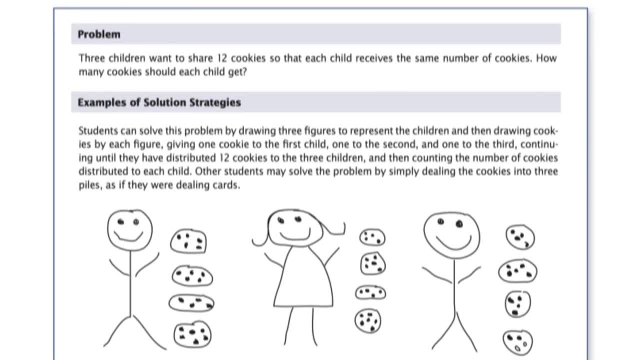 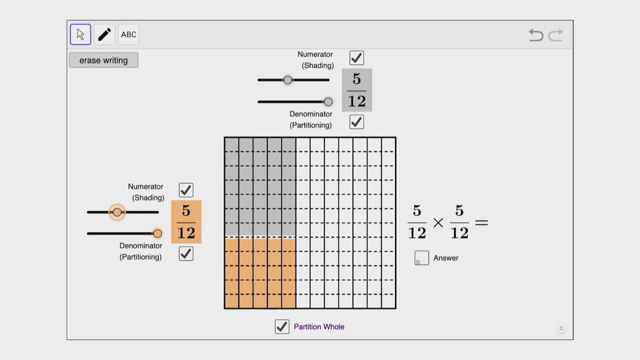 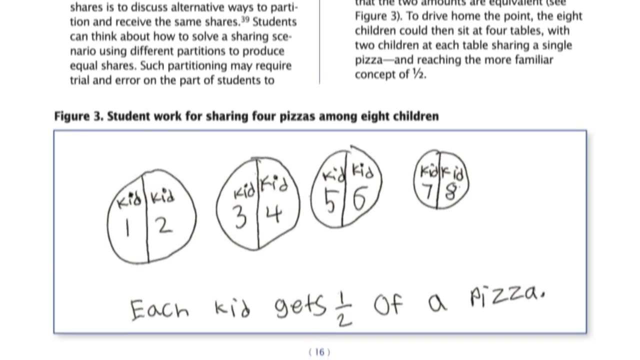 formative assessment prompts to help uncover misunderstandings, Interactive online applets that help them to see and build understanding of visual representations that are related to fractions, computation and ratio, rate and proportion, types of problems, as well as supports for teachers to 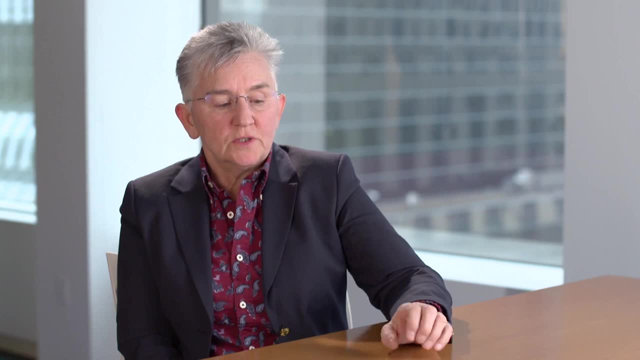 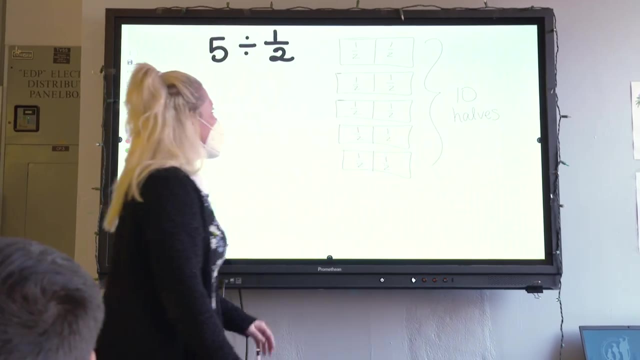 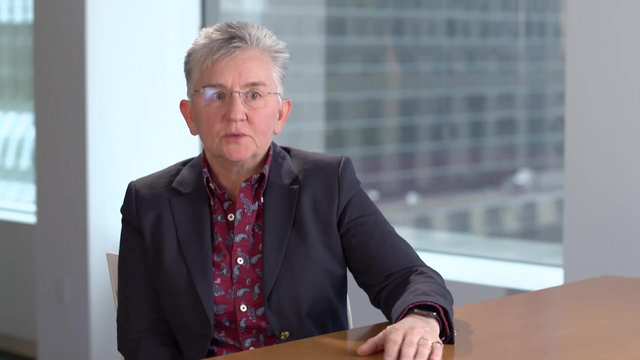 enact them in the classrooms. One of the things I think that's really helpful is having students have access to examples that are real life examples, Some guidance for teachers and being able to really have students understand conceptually what's going on with computation of fractions. 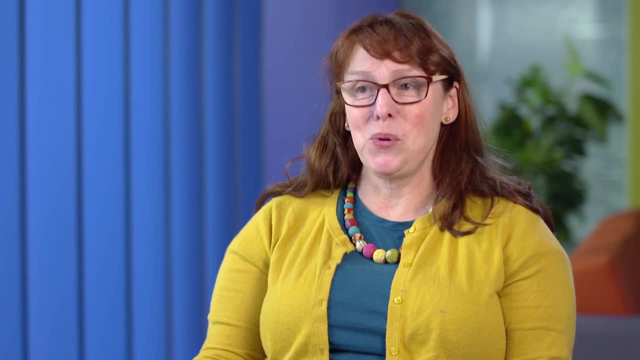 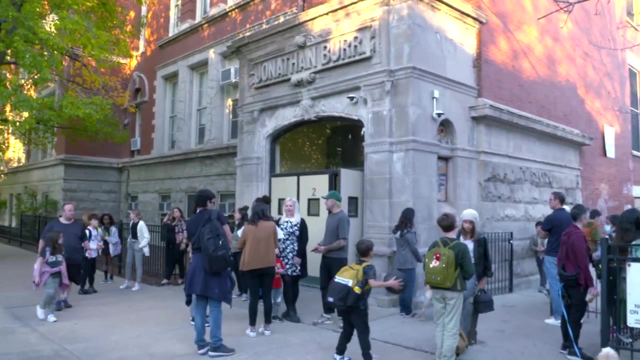 It always bothers me that people almost see it as a point of pride to say I was never any good at math. They would be appalled to say that about reading. You never hear people say, oh, I was never any good at reading. 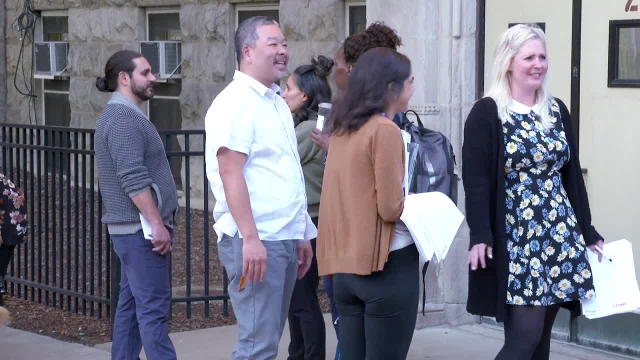 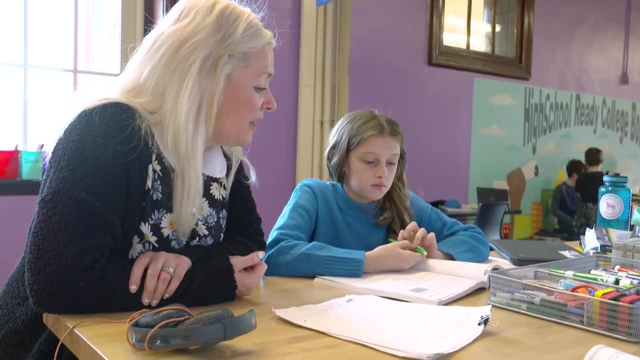 It's always math, But math is everywhere. We're a very data and information driven society. So even if you don't feel like you use a lot of information, you don't feel like you use math every day, And I think people tend to think using math means I'm. 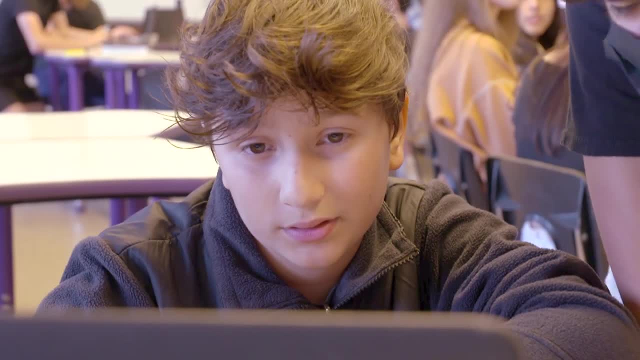 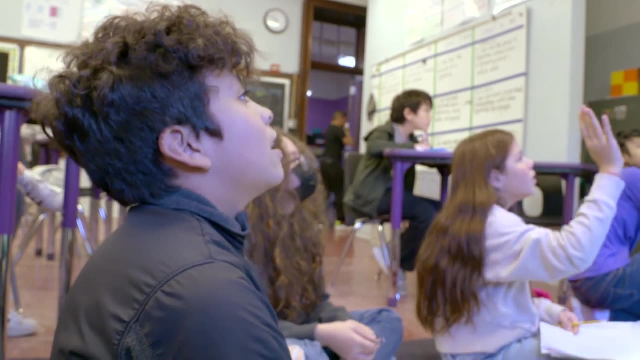 going to sit down and work these math problems. It's more being able to take in information, understand it, do something with it, And everybody needs to have that skill. Everybody needs to be able to interpret the information they're given, make decisions about it. 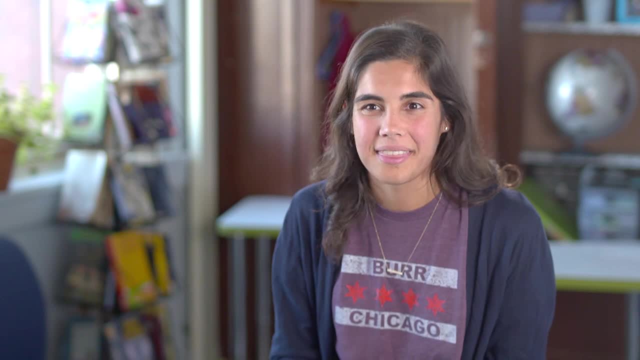 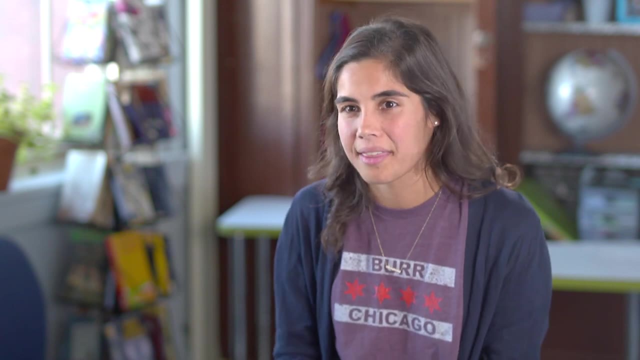 and do something with it. Confidence in math is definitely something that I think a lot of students struggle with, especially in middle school. A lot of them have that connotation that I'm bad at math or I can't do math. My goal with students is to be able to use math.